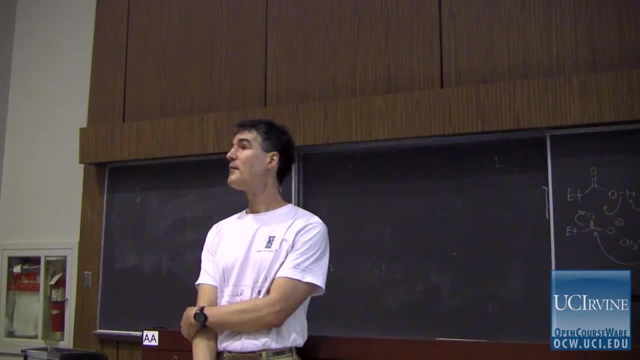 You actually talk with somebody who's a pro at something, they sometimes can't tell you how they do it. Ask Michael Jordan how he does that acrobatic move And he says, yeah, I'm at the top of the key and I see an opening, and then it's in No memory of how it occurred. 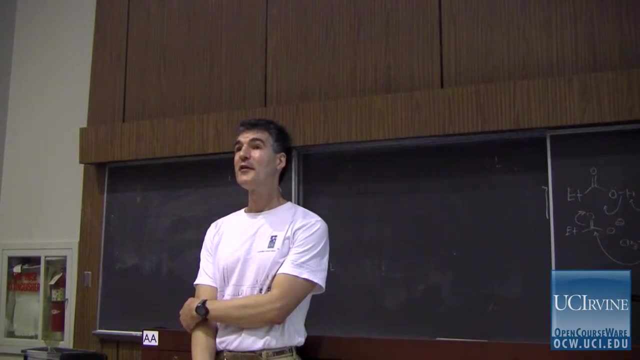 A person like that's not a very good coach, unfortunately, because you do need somebody who remembers what it's like to not know. I pretend very hard to do that, but sometimes it's hard to pretend, So if I go too quickly. 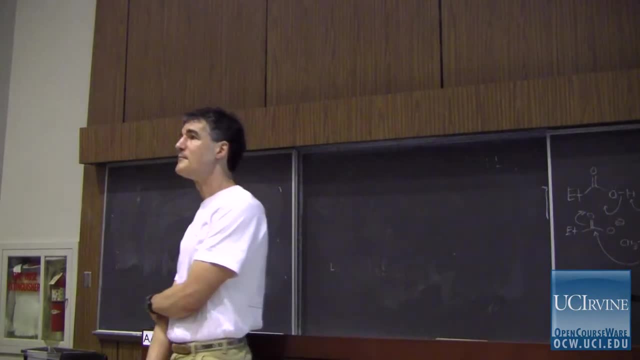 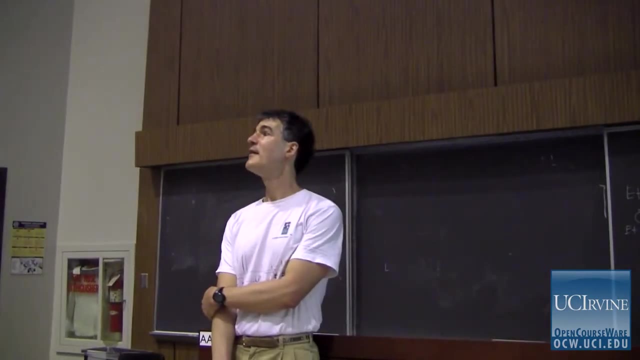 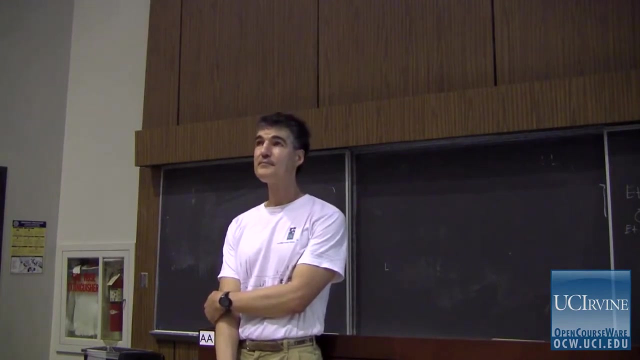 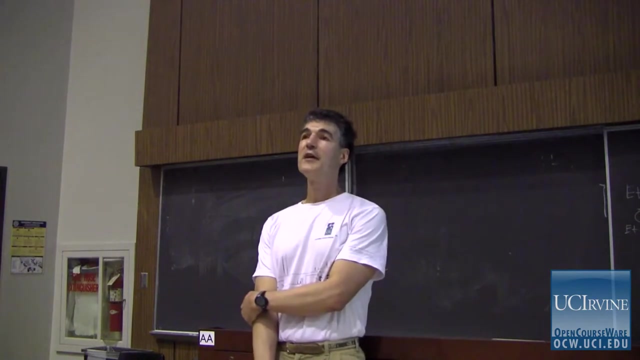 just ask a question. I don't mind clarifying things. I may think something's obvious, You may think everybody else thinks it's obvious. It isn't obvious until you know the answer. Okay, Now there is a very important characteristic to have during an exam, and that is mind control. 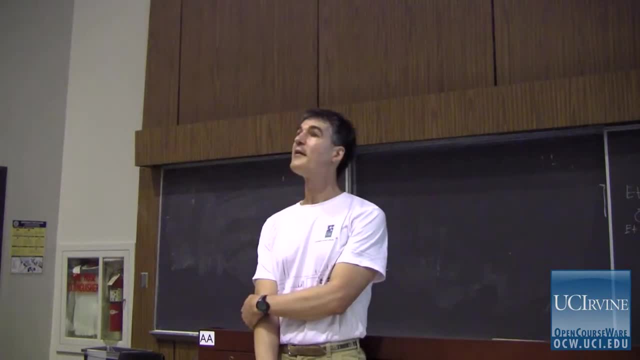 And that can be practiced as well, And I think it's worthwhile for us to take one minute and we will practice it. Here's what we're going to do. It sounds easy: We're just going to close our eyes, Breathe naturally, And when we breathe in, we're going 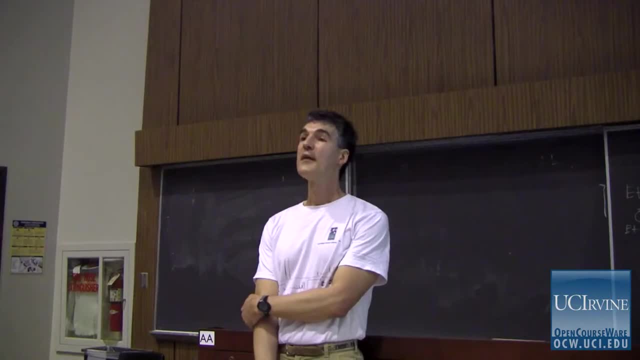 to mentally count one. When we breathe out, again we count two. When we breathe in, again we count three, And when we breathe out again we count four. And then we keep repeating: one, two, three, four, Ready, Let's try it for a minute. 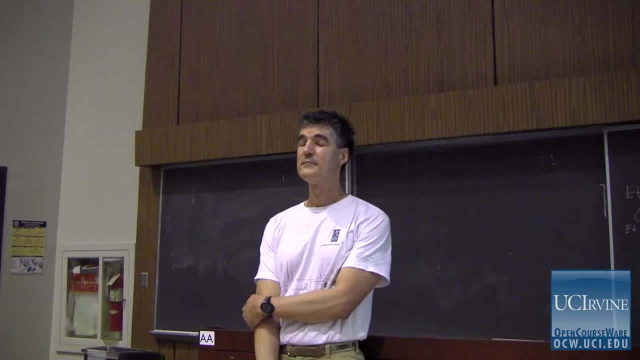 Okay, Start with your core. push your palm to the center of your forehead, use your chest as well. Huh, Let's start with the butt. put your foot into a cycle and then pull towards the top. You are bars. 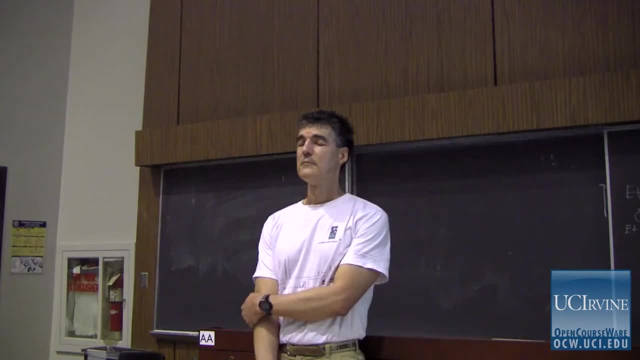 Thank you. Okay, That's a good way to prepare for an exam. Most people can't control their thoughts at all And they don't even know they're not controlling them. One, two God, this is a waste of time. 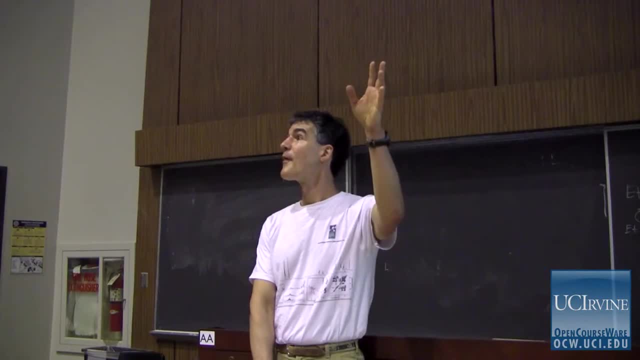 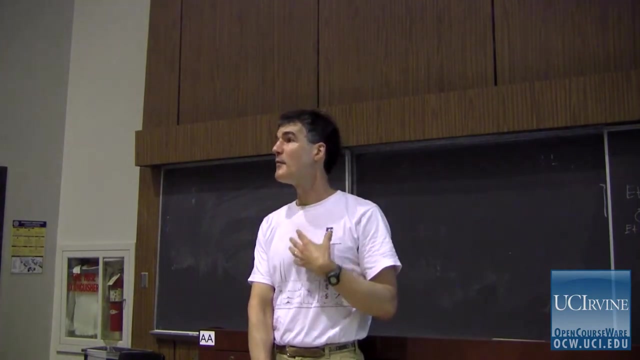 What happened? You find yourself thinking about something else, Listening to somebody coughing. What happened to three and four? Then you have to come back, And then you may be able to stick there for a minute. and then something else. I gotta go shopping. 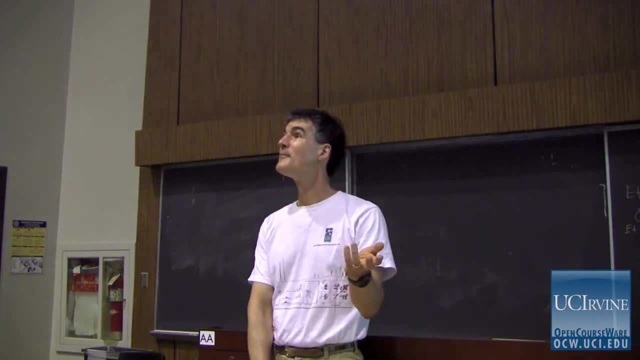 Where'd that come from? You notice that you don't know where those things are. Those things are, Where do those thoughts are coming from? And they're distracting, And the more distracting thoughts you have come in when you're trying to solve a problem. 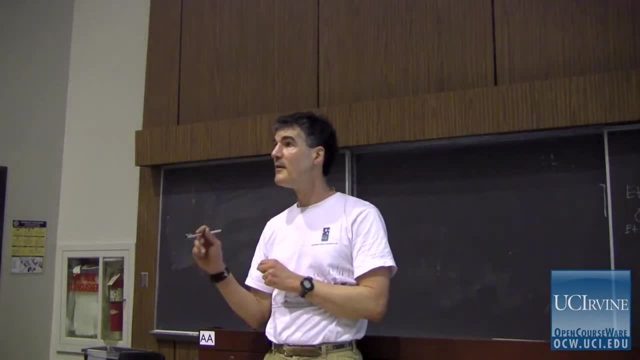 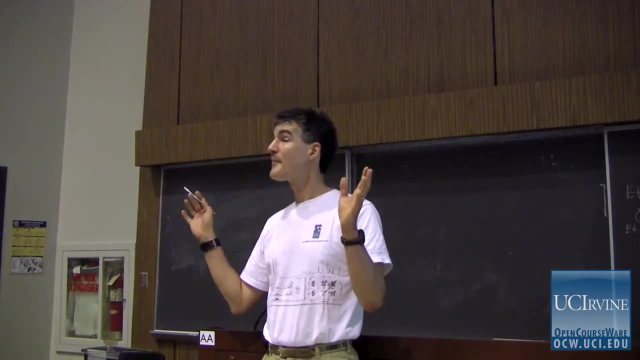 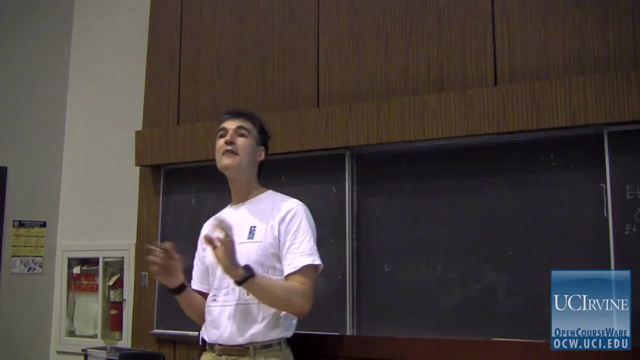 Let's see P plus AN squared over B squared. Jesus, I'm gonna flunk. What happened to the problem? Okay, It's possible to be in a low-grade panic for two hours during a final And never get anything done. 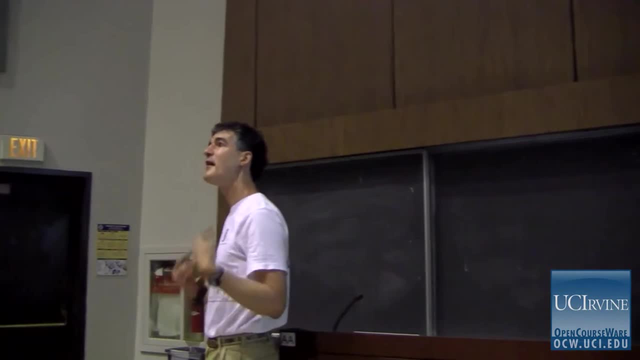 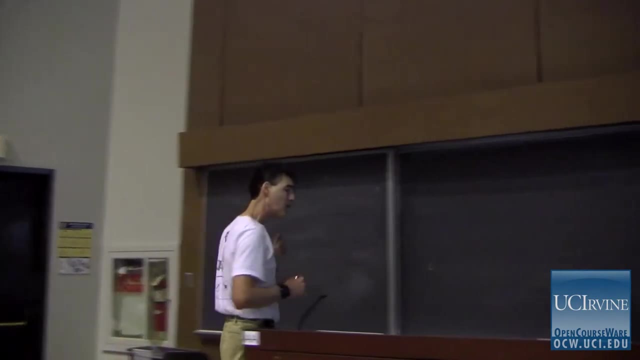 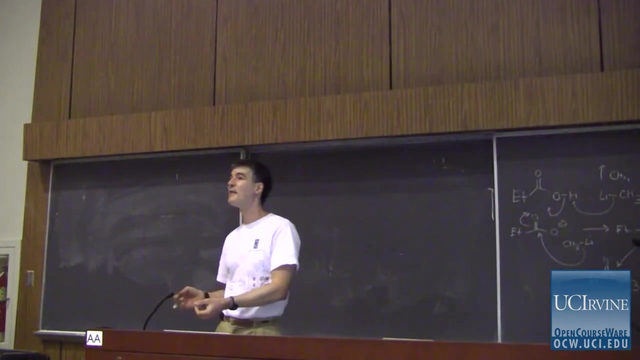 Because you're undermining yourself all the time with thoughts of failure Or triumph, But not thoughts or self-doubt. I should have studied harder. I'm no good. I knew this problem was gonna be here. There's three thoughts that did not help you. 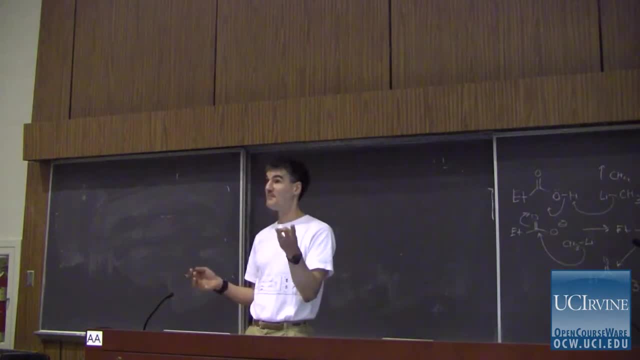 solve the problem And wasted time. If you want your life to go by just in the wink of an eye, spend all your time thinking: Be preoccupied. The more time you do that, the more the day will just disappear into nothing. 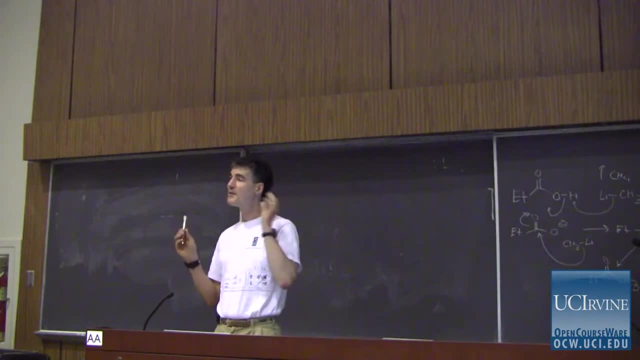 The more time you spend in the one, two, three, four mode, the longer your life will be. Okay. And if you watch those distracting thoughts, the longer your life will be. And if you watch those distracting thoughts, the longer your life will be. 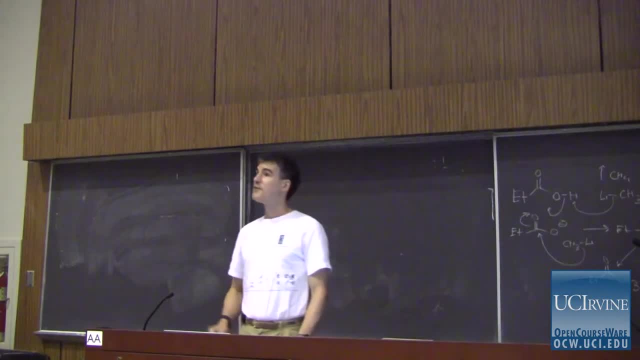 Okay, And if you watch those distracting thoughts, the longer your life will be. And if those distracting thoughts come up, then you'll dismiss them during the exam and get back focusing on what's important, Which is just how do I solve this problem here? 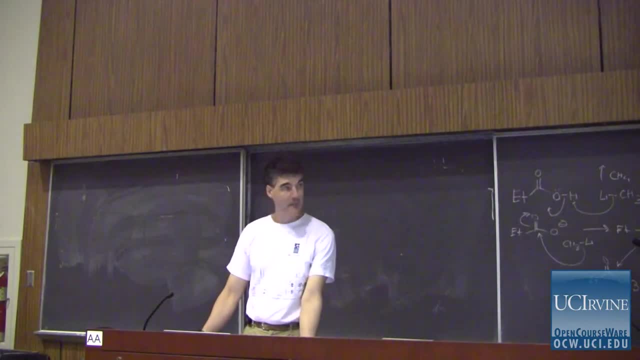 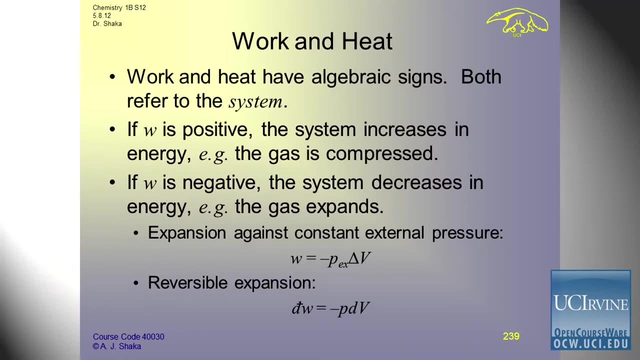 Okay, Let's talk about thermochemistry, work heat, enthalpy and heat capacity. today Quite a lot on our plates. Work and heat have algebraic signs. Both can be positive or negative, And both work and heat refer to the system. 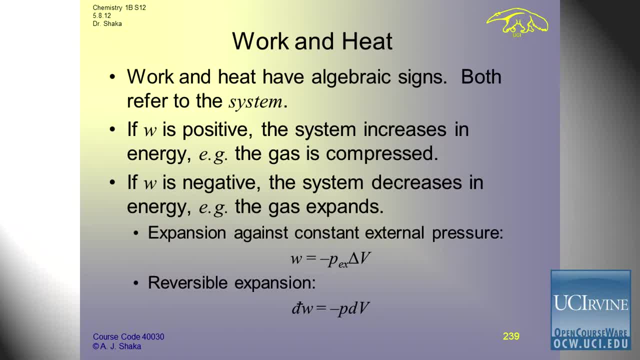 which is that part of the universe that we've mentally carved out to study, And the rest of it we call the surroundings. And we aren't quite as interested in the surroundings, Just like a person who owns property is interested in the property up to the fence line. 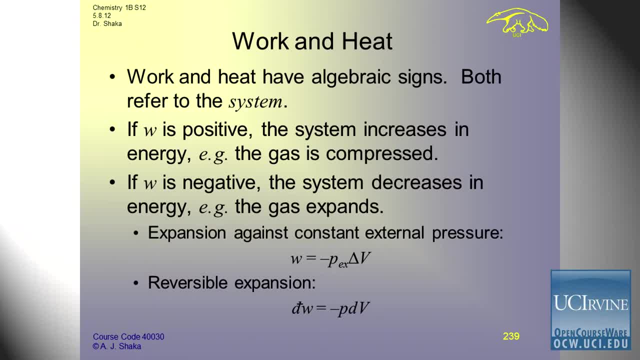 and then not quite as interested in the millions of acres beyond that they don't own. If the work W is positive, that means the system increases in energy. The system increases in energy. That means, for example, a gas is compressed. We have to 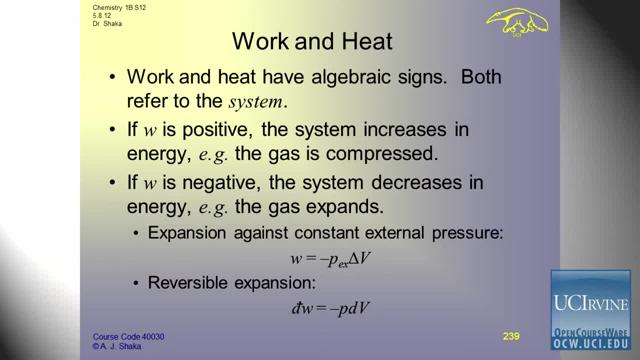 do the work to increase the energy of the system. If W is negative, the system decreases in energy and the gas expands. If we have a system like a power plant, where we're using the system to produce energy, we want the system to do negative work, so that 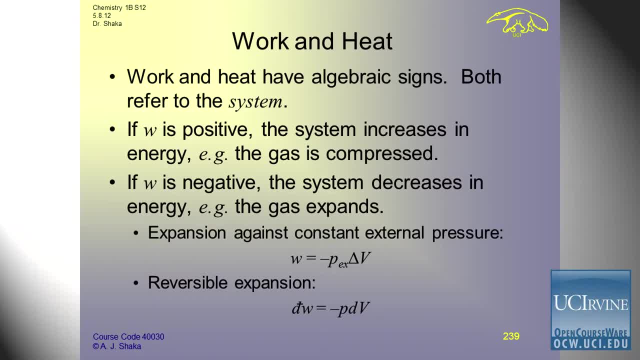 we get the work And we get to use it. So the energy of the system goes down and we get the energy to drive our car or do something else with it. And if we have expansion against a constant external pressure, then the work is just. 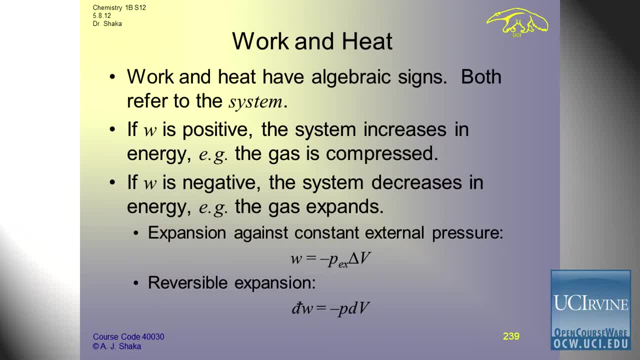 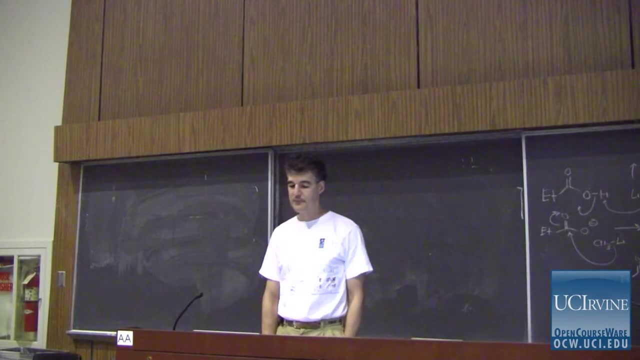 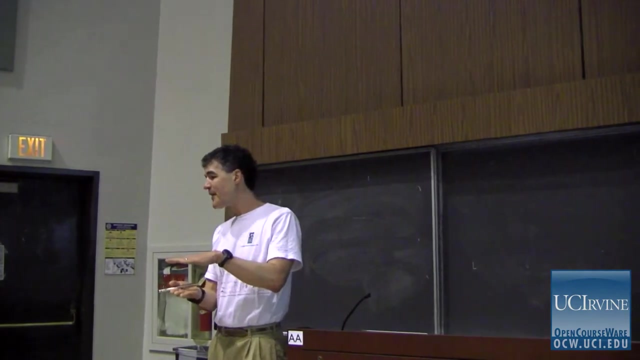 minus the external pressure times the change in volume. If W is positive, then the work is negative. That means the system expanded and so its energy is less, And if we have a reversible expansion, that means that the external pressure is always essentially the same as the internal pressure. 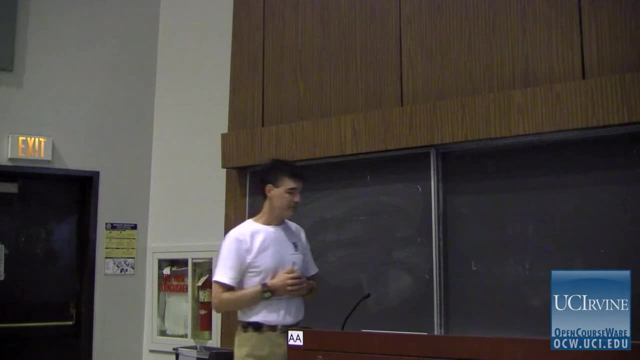 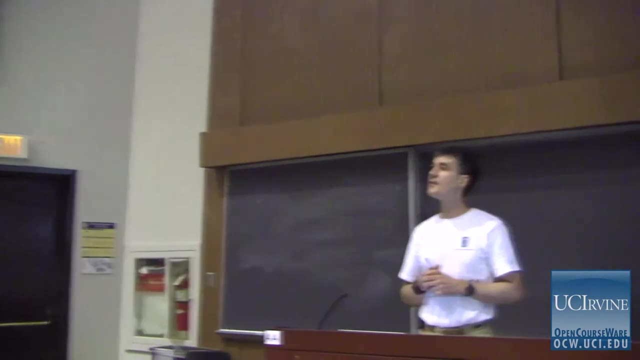 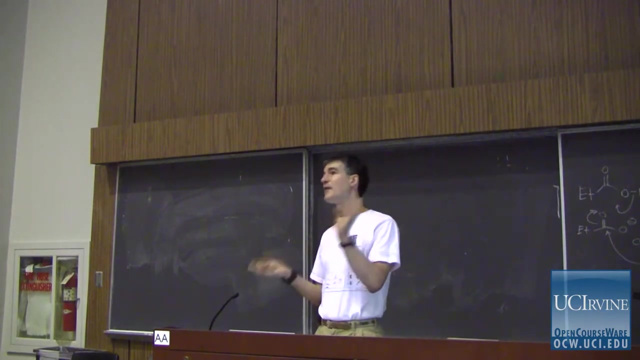 So that it expands ever, ever so slowly, and that means that we can just use the internal pressure. The reason we like reversible expansions and reversible things is that they're simple to figure out. It's not that we're ever going to do them, It's they're simple to figure. 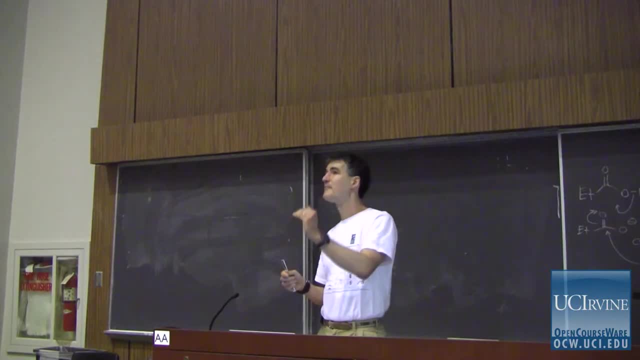 out and they tell you the best you can possibly do. You're always going to be worse than that. If you're not good enough, you've got to do something else. That's very important to know what that limit is. So reversibility again. 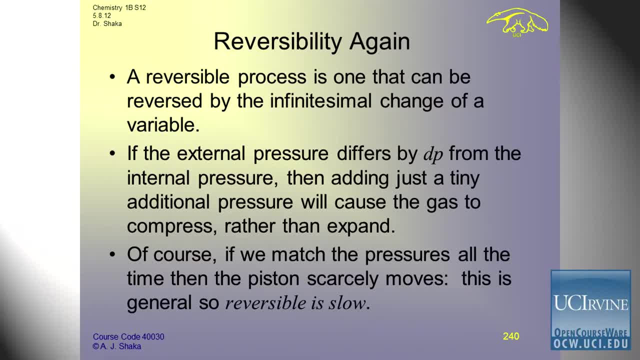 we've gone over this. but a reversible process is one that can be reversed by just changing an infinitesimal amount of pressure. if it's reversible, then it starts to contract again, So there's a little bit extra pressure on. So it's essentially matched. 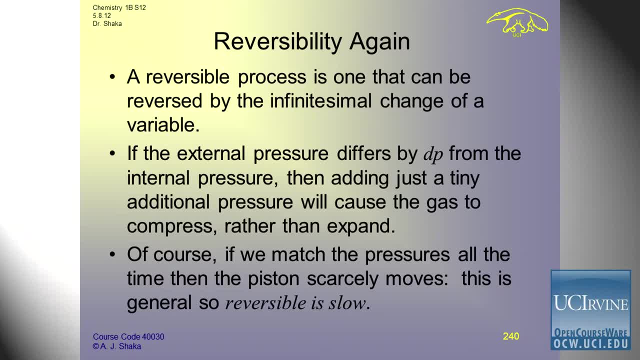 And the beauty of calculus is that you can have something differ by such a small amount that it's essentially zero, but it's not. It means that you can do an integral, And integrals, as I will show you, are easier to do than some. 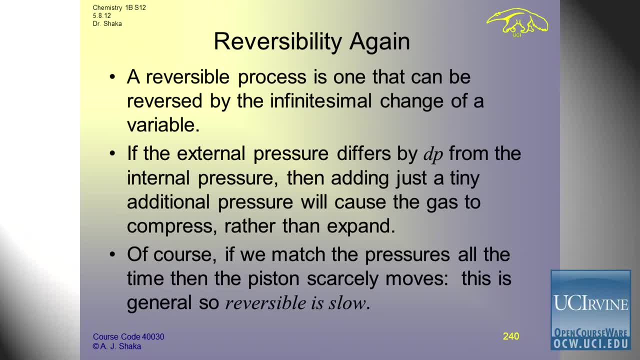 And the reversibility is always extremely slow. In principle it's infinitely slow, So we can't possibly do anything reversibly because we can't wait. that long Time is money. More importantly, we all live for a certain amount of time. That's why very few people plant up white oak, Because if it takes 400 years to mature, you have to really think way far ahead beyond what it takes to plant it. Most people plant a tree, like a eucalyptus, that grows like crazy and doesn't live as long. 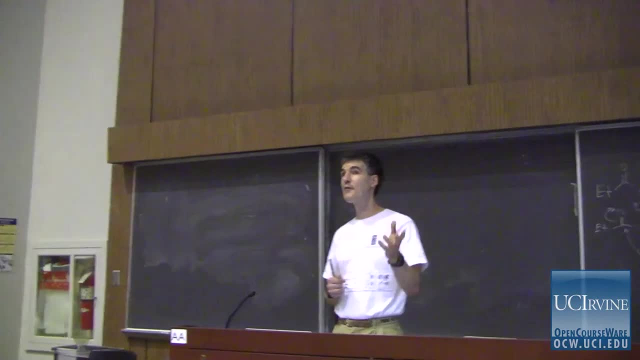 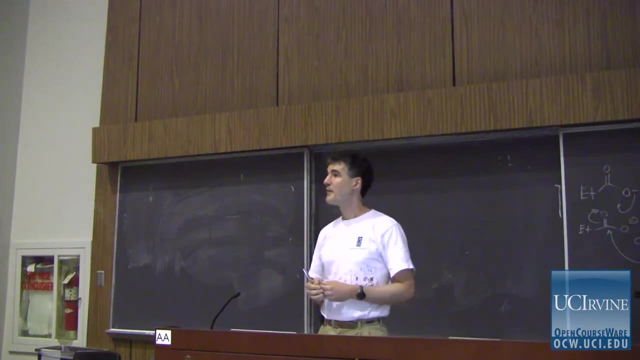 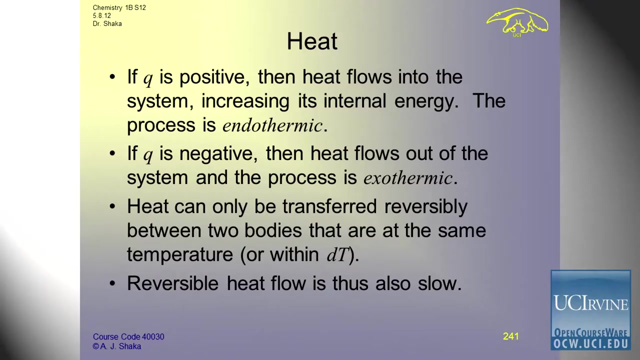 so that it will be big in their lifetime. That's why we need some kind of programs where people look further ahead to the future for the common good and just plant things like that so that future generations can enjoy them The same thing. if Q is positive. 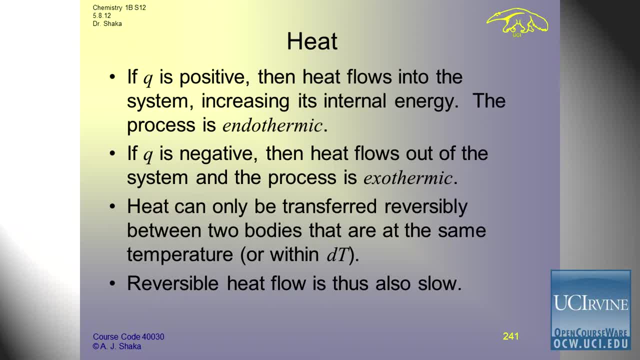 then heat flows into the system and increases its energy. That kind of process is called endothermic. It absorbs heat from the environment. it's going to feel cold, It's going to be a kind of reaction that tends to get cold and then absorbs heat from the environment. 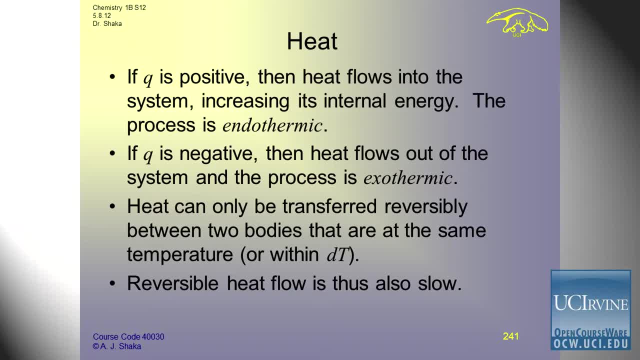 to warm back up. There are favorable reactions that do that. but I think, for example, if you dissolve ammonium nitrate in water, it gets cold, It still dissolves. I think early chemists thought that every favorable reaction that would just occur on its own. 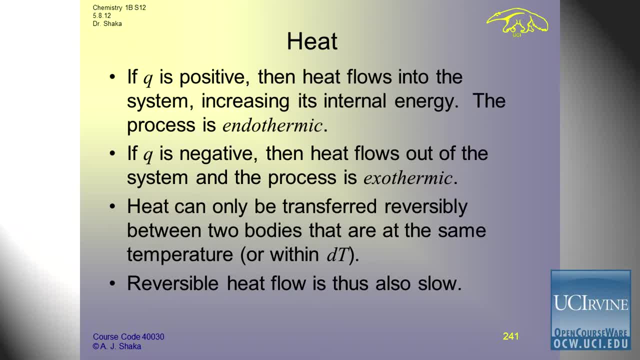 produced heat, And that's broadly true. Many of them do like burning gasoline or wood or many things that it's just down to heat was wrong. If Q is negative, then heat flows out of the system and the process is exothermic, And that's the kind of thing. 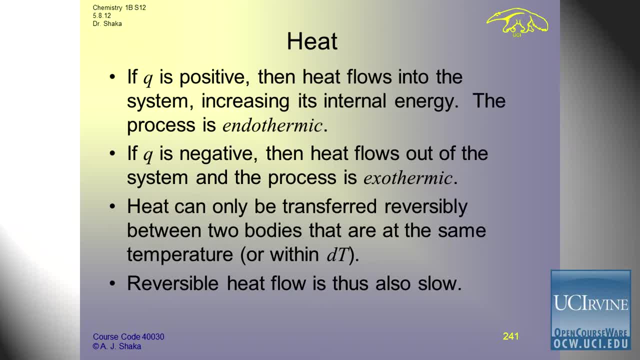 that we use to create power. We run exothermic reactions and then we use the heat in some kind of a heat engine to produce work, For example, if you have a fire- and you have a fire, for example, to spin a turbine and generate electricity. 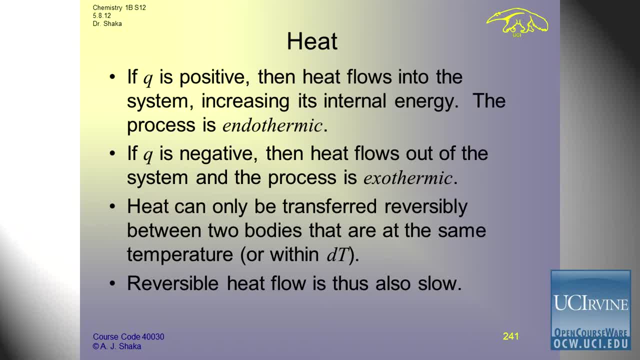 we burn coal, we produce heat, we produce steam, we produce work, we produce electricity and we produce a ton of CO2. unfortunately, Nobody thought that was bad when the industrial revolution started. Heat can only be transferred reversibly if you have two things at the same temperature. 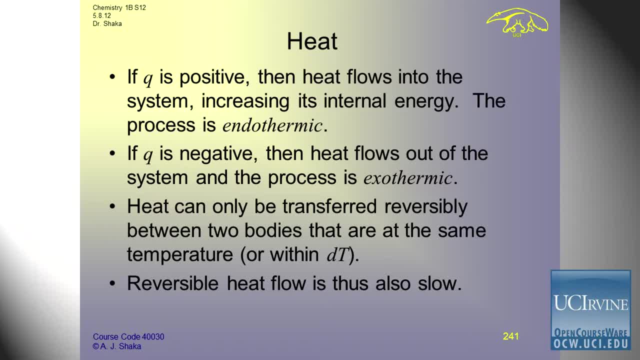 or within DT. Once two things are at different temperatures, if you bring them into thermal contact, it's over. You've just lost, Because the heat goes from the hot body to the cold body and then you can't get it back. You can't magically. 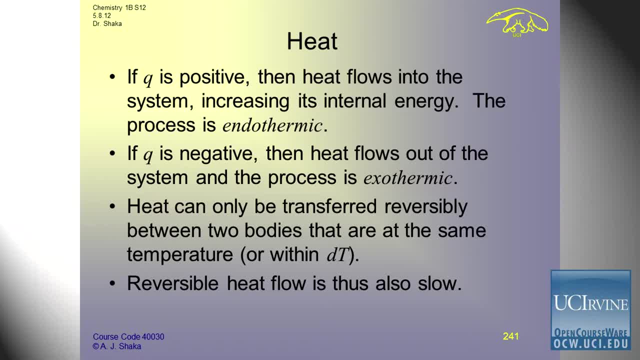 separate heat by just waving a plastic wand. But you certainly can take boiling water and ice and you can mix them together and you get water at some intermediate temperature. That'll happen, naturally, And you can see microscopically how that happens, because the boiling water hits the ice. 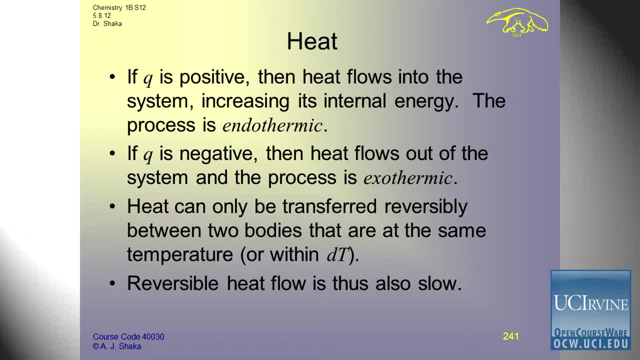 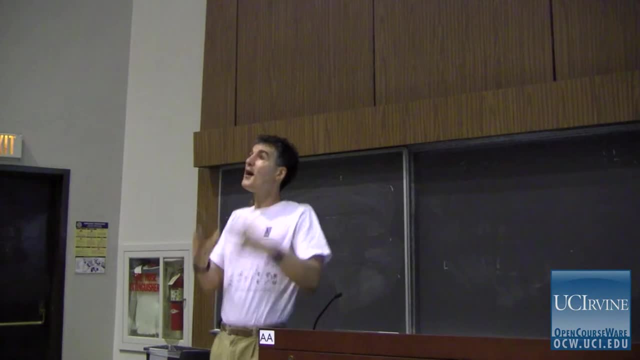 and then knocks the water molecules out of the ice And then they're all there and they all settle down and that's all that can happen. It's the most likely thing. It's very unlikely for part of the water to suddenly stop moving and freeze into ice. 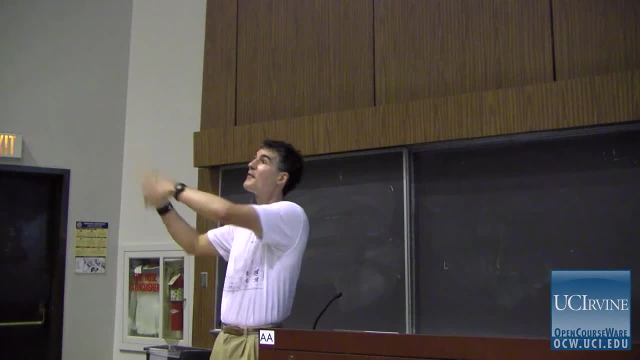 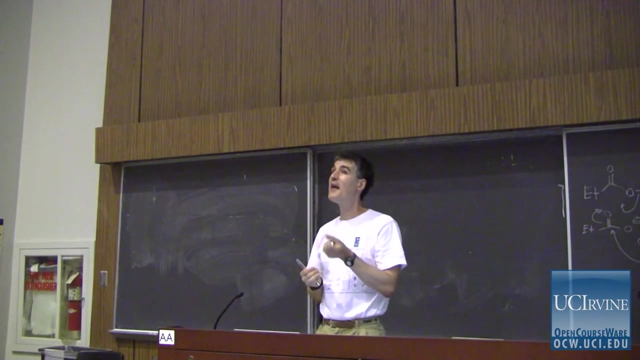 and transfer its energy magically to a bunch of other water that's moving fast and suddenly boiling. That's extremely unlikely, And so we don't ever see that happening, Although many of the greatest frauds in science have been to propose a machine that essentially 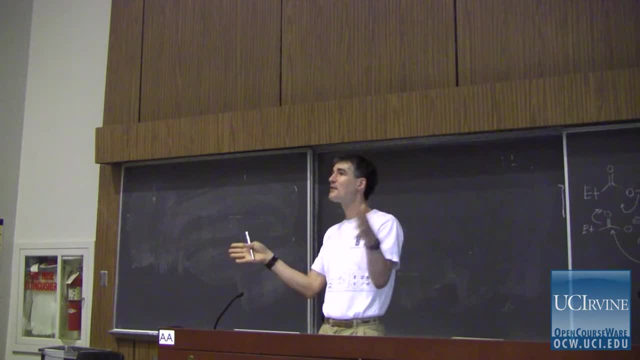 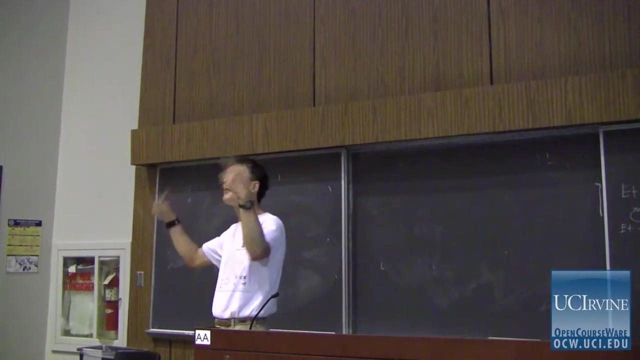 does that Separates heat into two parts, a cold part and a hot part. and then you run something with the hot part. So you have a submarine, you're going along. you just take in sea water, you chunk out ice cubes out the back and then you create steam. 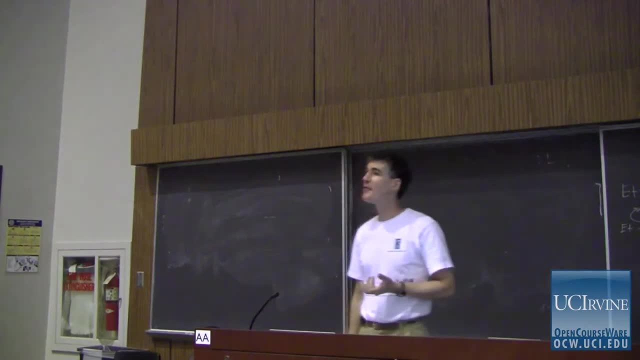 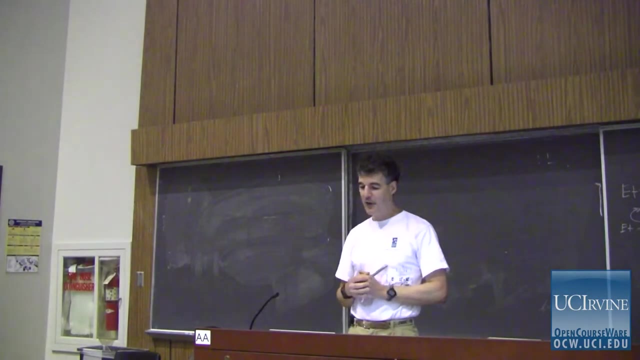 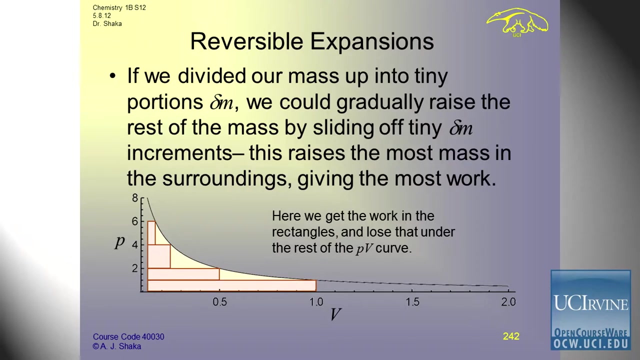 and then you power the propellers of the submarine and that stuff won't ever work. Reversible heat flow- if they're essentially at the same temperature, is also slow. Okay, Remember we had that piston and we pulled the masses off. we had four and we slid them off. 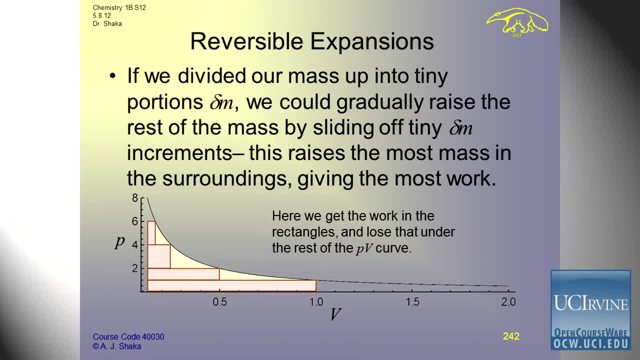 when we got work and if we slid them off more slowly than we can and just flicked them off, then we'd end up with the most sand piled up the highest and we'd get the most work. And here, if we have four masses, then initially, 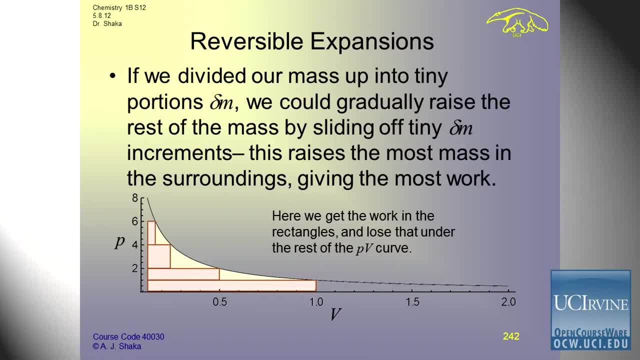 we pull a mass off and the pressure goes down from six to four and therefore it expands until it hits this curve, which is the PV curve- and remember, if it's at constant temperature, PV is a constant because it's NRT- and then we pull another mass off. 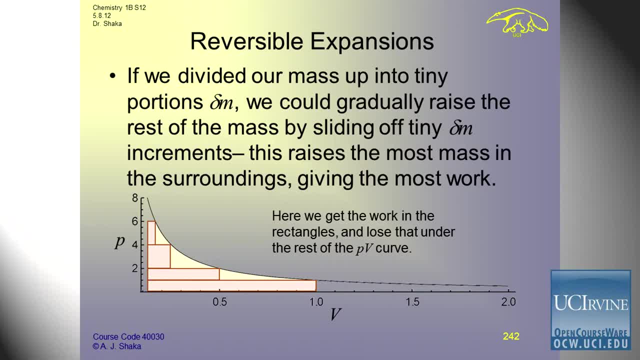 and it drops to two. let's say: and then it goes out to here and we pull another one off. let's say, it drops to one, goes out to here. we capture then the stuff in the pink, we get the work in the pink and we lose the work in the yellow. 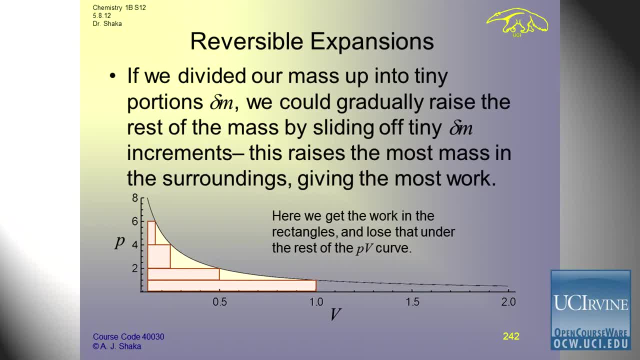 and so we say: gee, if we wanted to capture this thing, we'd have to drop it down maybe to five, and then it would go to here and we'd carve out a little bit bigger rectangle, and then, if we did it even more slowly, we'd go like this: 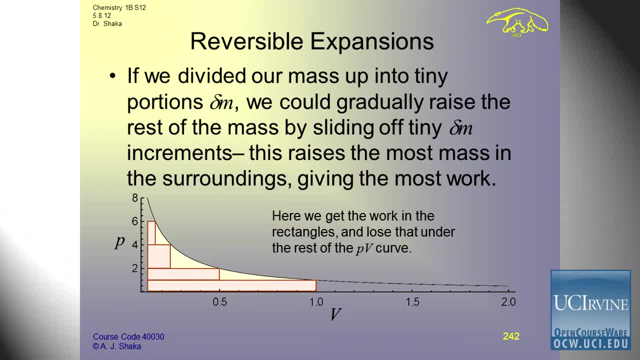 and then finally we'd get this curve, as if the external pressure is just the pressure of the gas at all times. and ironically, the area under this curve is a lot easier to calculate than adding up these squares. especially if there's a lot of squares, that gets tedious. 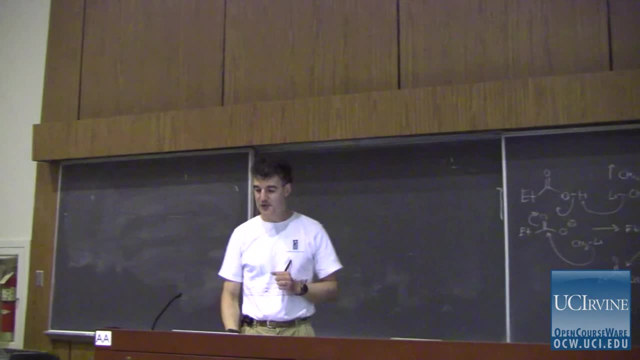 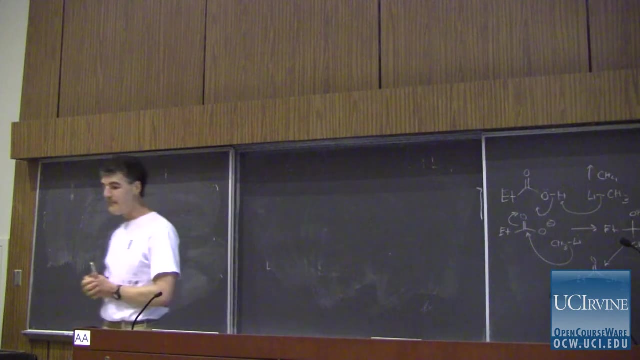 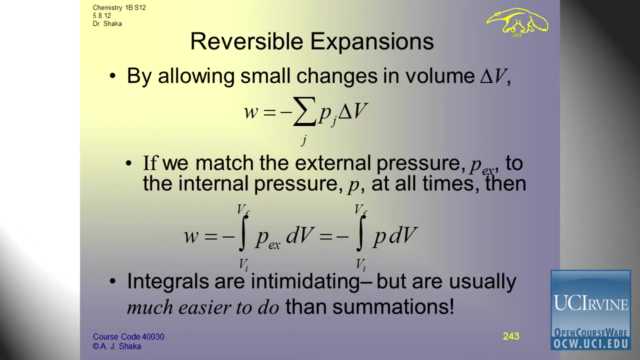 to do. the formulas for sums are tedious, the formulas for integrals are not, so this would be the sum. I take off mass, I adjust the pressure and I have to add up each change in volume times the pressure that was in effect at that time. and if this is hundreds of things, 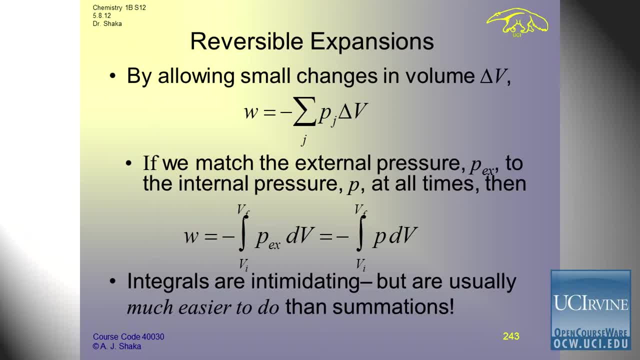 I have to add these up, maybe with a spreadsheet on a computer. but if we match it at all times so that we get this area under the curve, then this sum magically turns into an integral. and even though the integral is intimidating when you don't know what it means exactly, 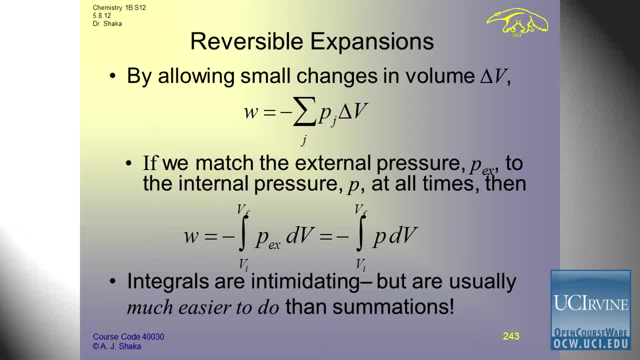 the integral is much easier to do than the sum, and that's why chemists love reversible processes: because they can just slap an integral, do it easily figure out what the most they can get is. you're not going to get that, so you have to work on what the efficiency is. 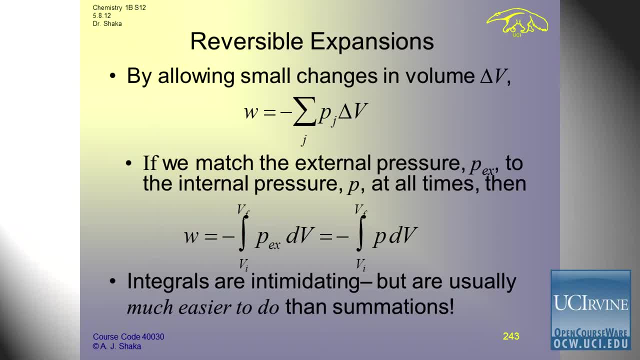 so we'll give an example here. the integrals look intimidating. in fact, I quite clearly remember when I was five or six- because I was still on the east coast- my father had a book that had all these things and he said: I want to learn, and I was absolutely. 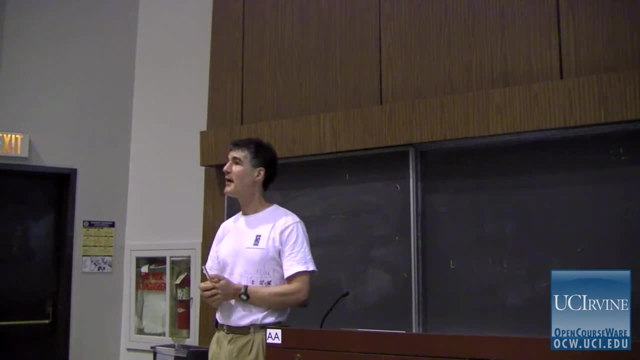 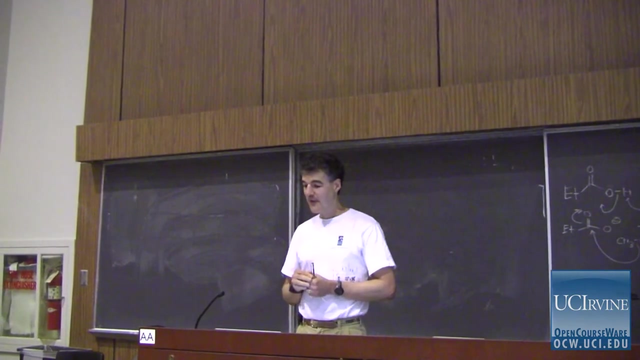 fascinated by that book and what those could possibly mean. and when would I learn what they meant? would I learn that in kindergarten? and my dad said, no, you won't learn it in kindergarten, but you'll eventually learn it, sadly. you may have heard Maurice Sendak, who wrote: 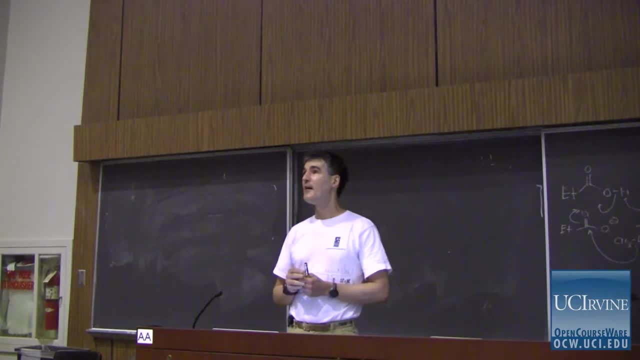 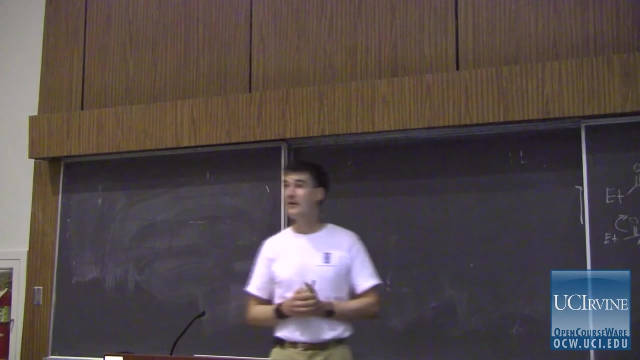 part of the wild things are: yes, will we have to know how to do it? no, but anyway, I can show you how to do them. there's a trick. Maurice Sendak died- he had a stroke, I think on Friday, at age 83. that's another thing. 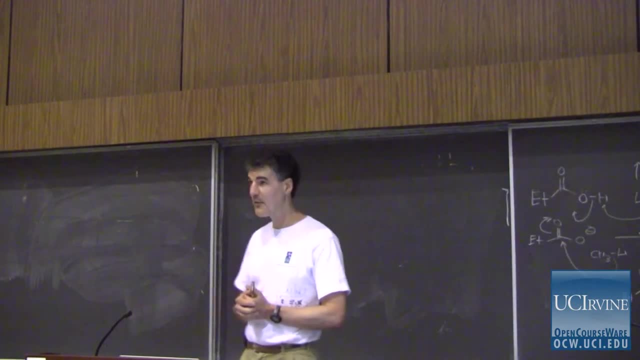 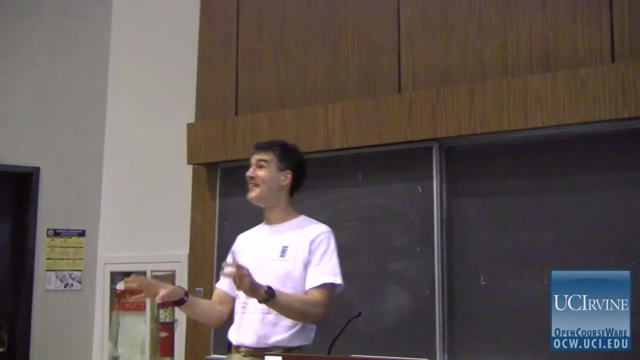 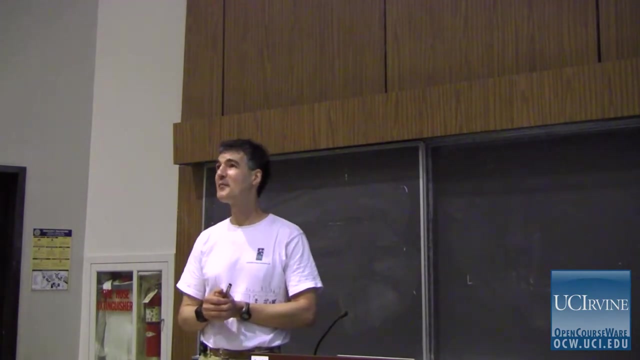 I clearly remember as a child as reading that book, and then I thought there are monsters because they're in the book. so you have to be careful. just because you can imagine something doesn't mean it's true, and even if you draw it, it doesn't mean it exists. 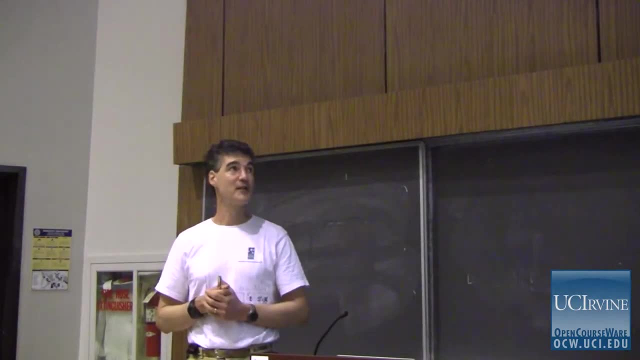 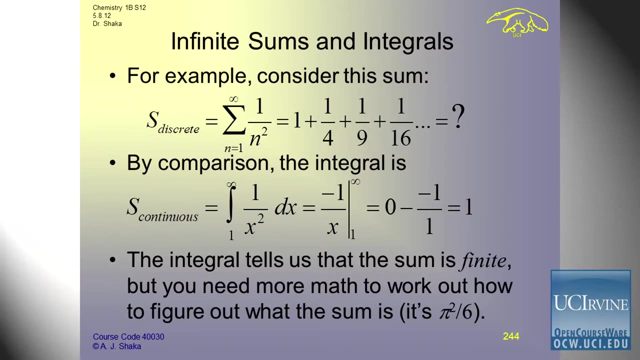 you have to verify these things. so here's an example. here's a sum: 1 over n, squared to infinity: 1 plus 1, fourth plus a 9th, plus a 16th plus a 25th, and the answer. the question is, what is that? 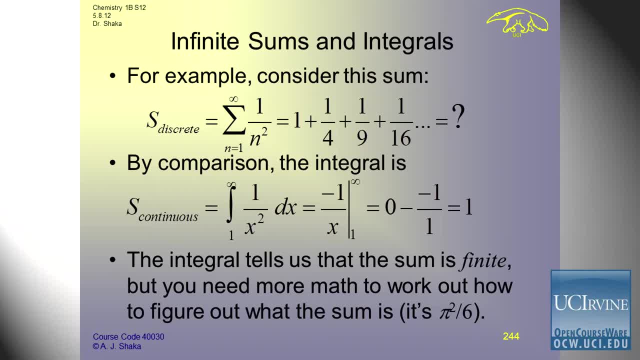 what is that total to exactly? so I can't just do it on a spreadsheet because it's got an infinite number of terms. so I need to stand back and use the power of the human mind, and the beauty is you can sum infinite numbers of things. computer can't. 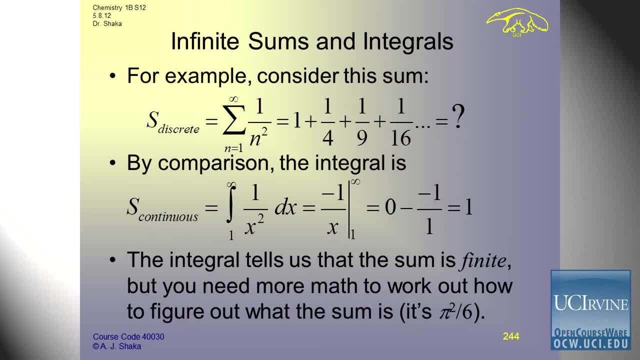 by comparison, though, the integral is pretty easy. the integral from 1 to infinity of 1 over x squared is: minus 1 over x, evaluated at x equals infinity. minus 1 over x evaluated at x equals 1. the two minus signs go away, so the area. 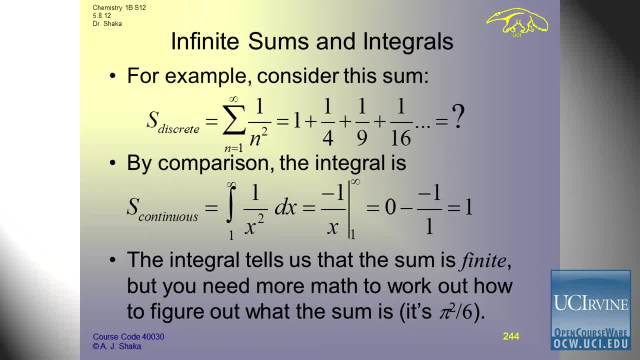 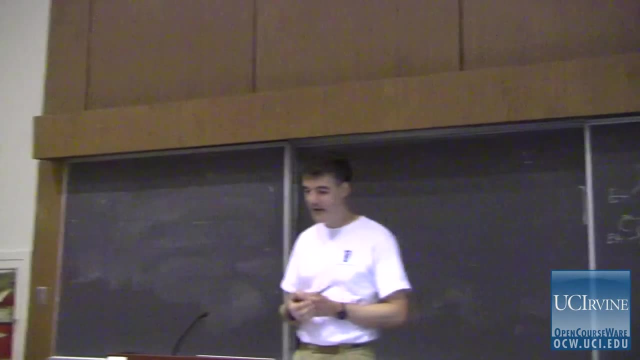 under this curve is 1, and this is going to be bigger than that, obviously, because this is outside the curve. before the rectangles were inside the curve, now they're outside the curve, and in a more advanced math class, you will learn, in fact, that that integral is pi squared over 6. 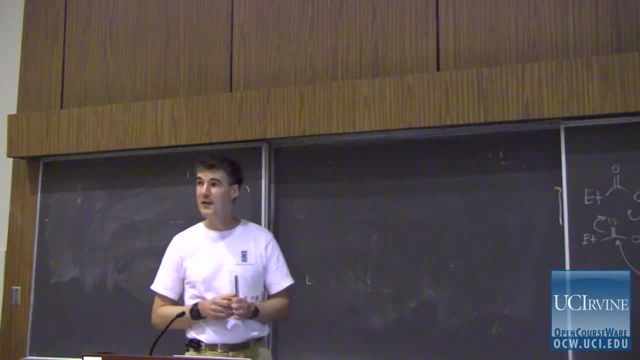 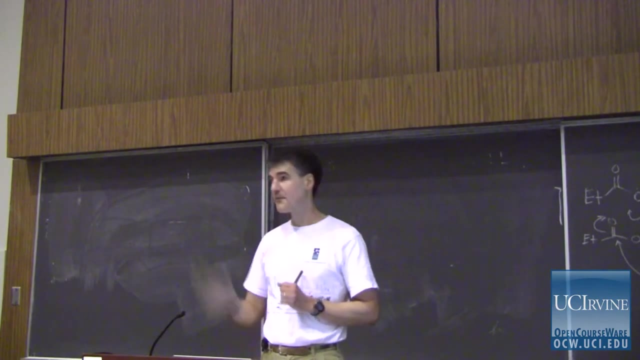 so you have to know something about Fourier series, but that's actually quite simple to calculate and that's what it turns out to be. so it's about 1.64, something, which is a number that doesn't look like anything. if you start totaling it, you can't guess what it is. 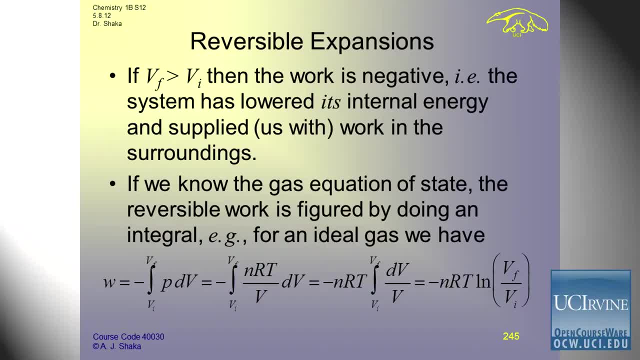 by the number. ok. if the final volume is bigger than the initial volume, the work is negative because the system has lowered its internal energy and supplied us with work in the surroundings. and if we know the gas equation of state, then we can figure out exactly what the reversible work is. 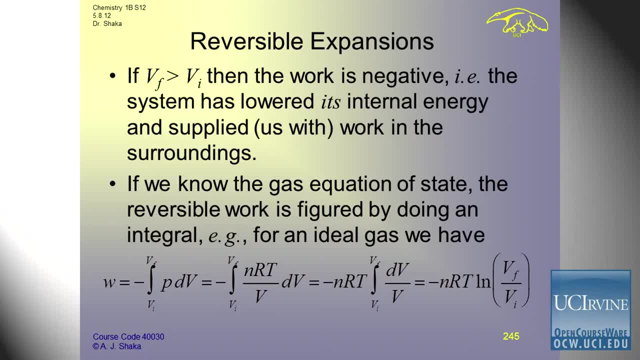 so if the pressure, external pressure- is just the internal pressure, I know what P is. it's nRT over V, nR and T are constants. there's nothing else here but V and dV. so I have minus nRT, dV over V, and that's the antiderivative. 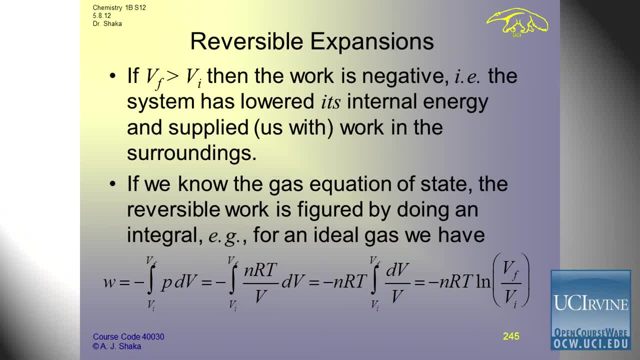 of 1 over V is natural log. so I get a simple formula here: minus nRT, natural log, plus 1 over V, initial. I want you to see these, but I'm not going to require you to do funky integrals on exams. this is not a math course. 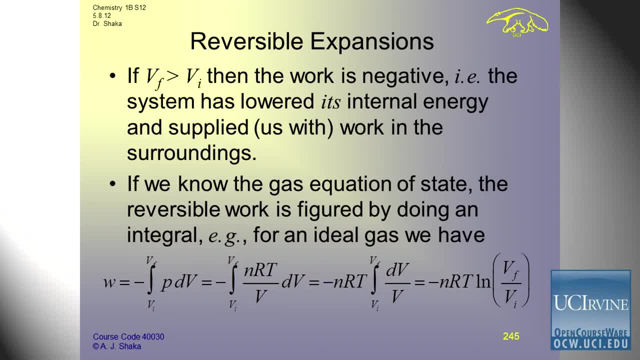 on the other hand, you mustn't be intimidated by things just because you don't understand them. now I found out recently that the Wright brothers knew nothing, basically nothing, about fluid mechanics. they just tried stuff in the history of engineering. oftentimes the engineers are ahead of the scientists. 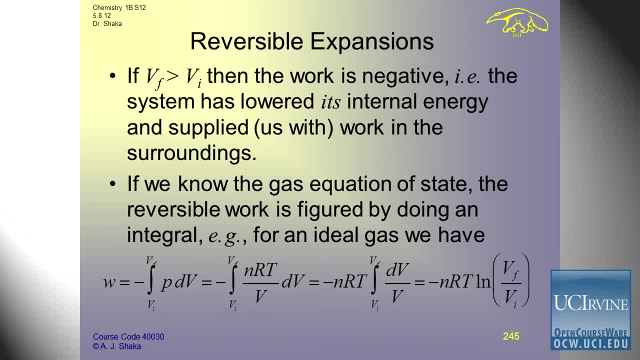 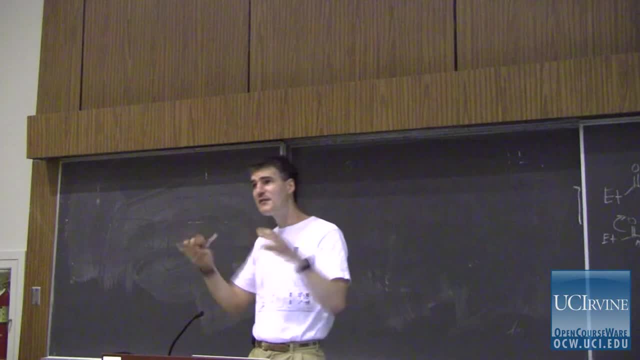 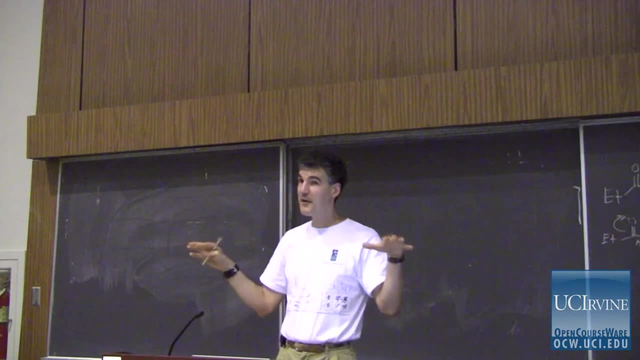 because they're just trying stuff and then they see what works, and then scientists come back and say: well, that means there's lift on the upper wing, and you should maybe adjust the wings like this and they should have this kind of curve on them, and so forth and so on. 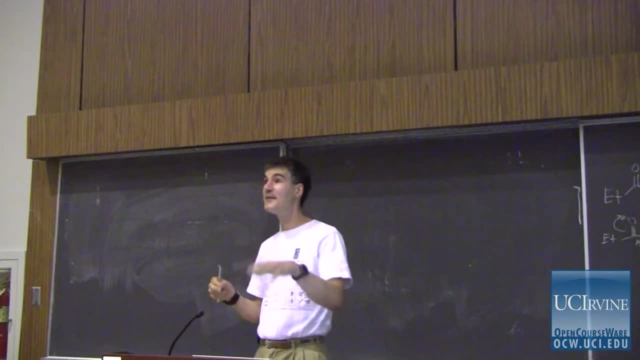 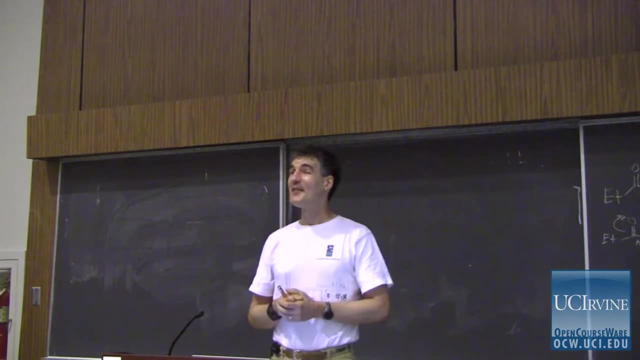 and they can improve it once they understand it. but you don't have to understand how it works to fly. if you're going to get in there, I don't know who you could have a bad accident right. just because you can get off the ground doesn't mean you're going to stay level. 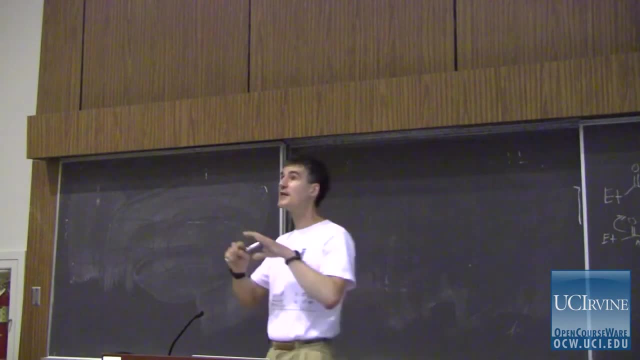 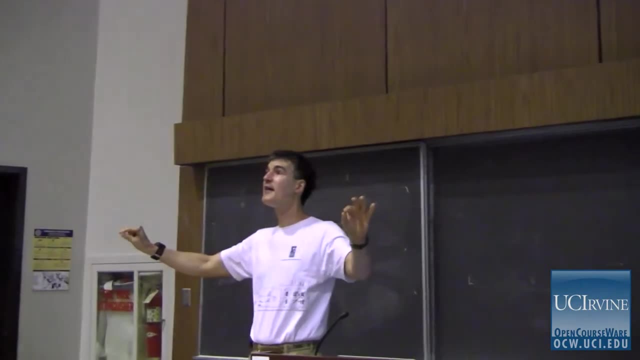 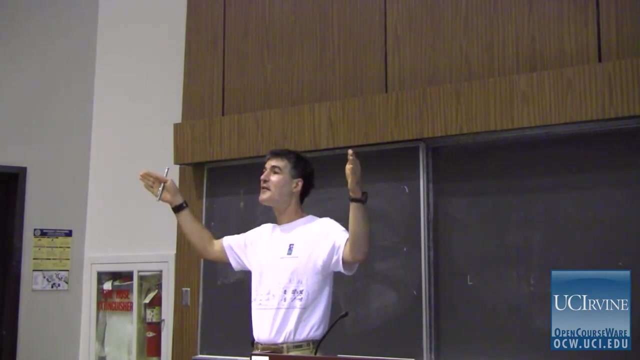 and, interestingly, for the longest time the wings looked like this. they came out on big jets, they came out like this, and then suddenly the wings started coming out like this, and then there's this little thing on the end and that turns out to give you much better gas mileage. 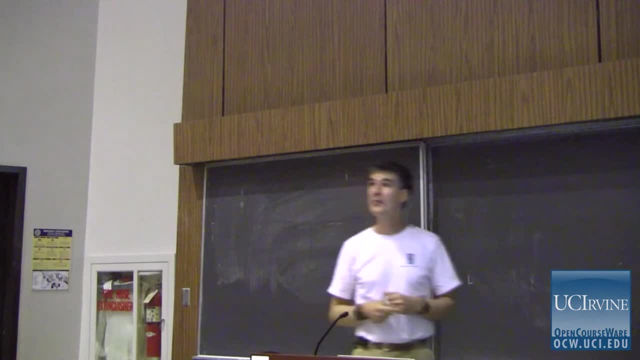 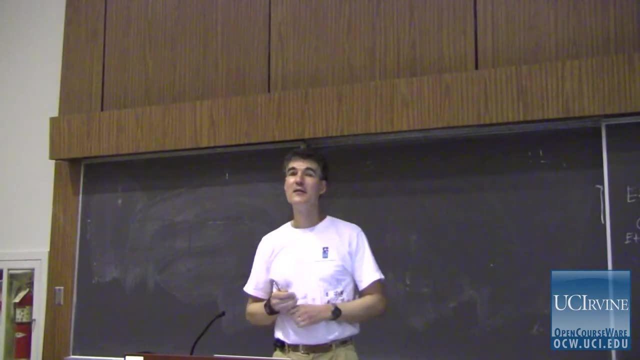 so you can actually model that. and some bright guy said: hey, if we just put this little thing scoop on the end, we're going to get much better mileage out of our kerosene. and then all the new planes have that now, because there's no reason not to do it. 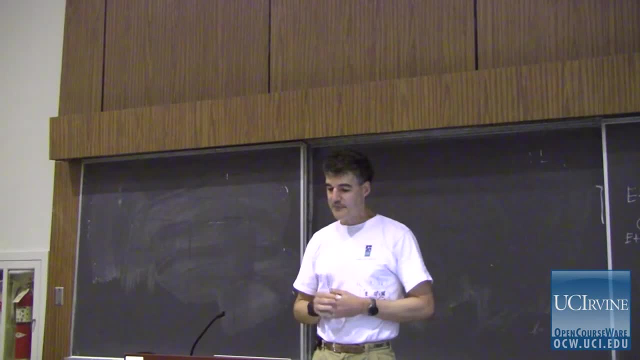 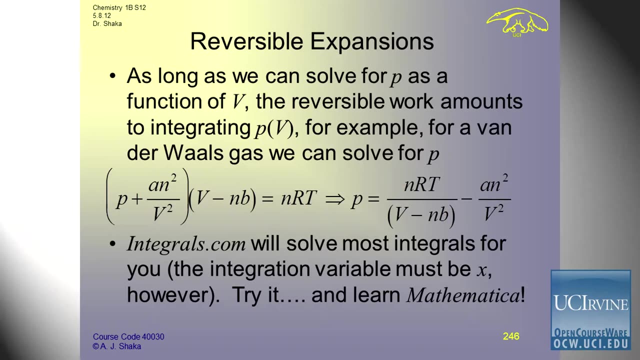 but they just haven't thought of it. so as long as we can solve for v as a function of v, we can do it. so for example, we can do a van der Waals gas here, because I can isolate p and all this stuff's v, and then I just turn this over. 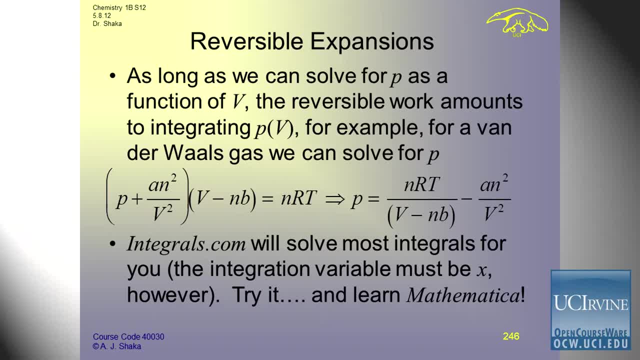 and put an integral on it. and in fact here's the secret: integralscom will solve any integral you give it. you don't really need to memorize the antiderivatives the way I did as a kid. that's one of the things I did. 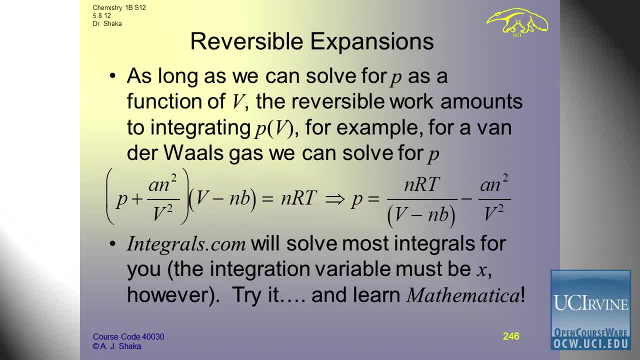 I memorized all the tricks, all the antiderivatives, tan theta, over 2 trig substitutions- you name it- so that I could do integrals quickly. because if you couldn't do integrals quickly, it's like having to look up every word in the dictionary when you're trying to. 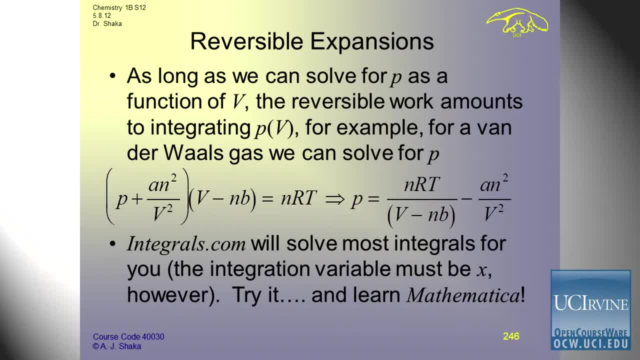 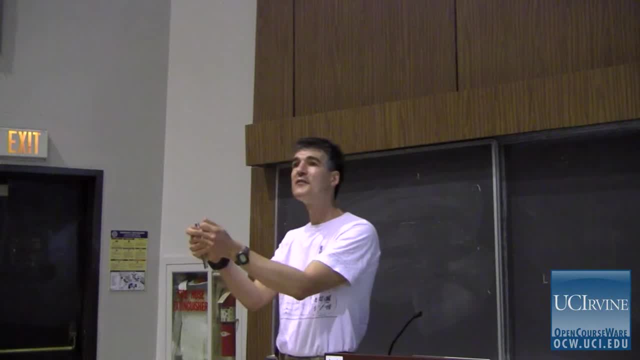 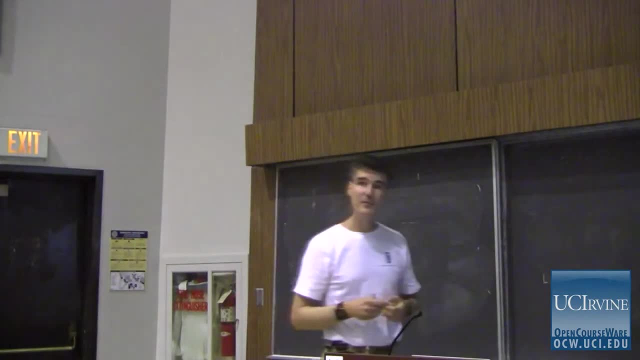 read Shakespeare, you can't get the flow of the play or anything, because you're bogged down. what's the definition of this? what's the definition of this? you can't get any flow and if you're doing lots of problems in physical chemistry, you can't see the problem. 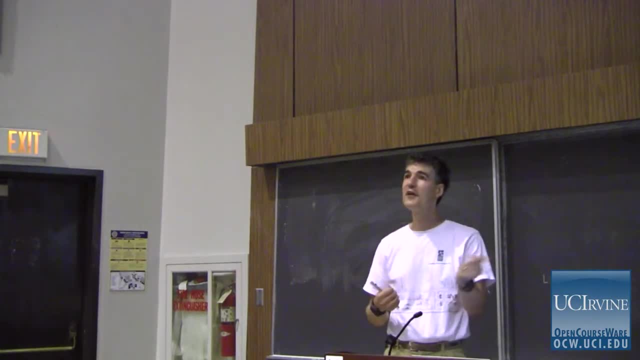 if you waste too much time getting stuck with the integral, so you just have to know the integral and then you keep moving. and it's like running: there's a certain pace at which it's comfortable to run. if you run too fast you get tired out, but if you deliberately try to run too slow, 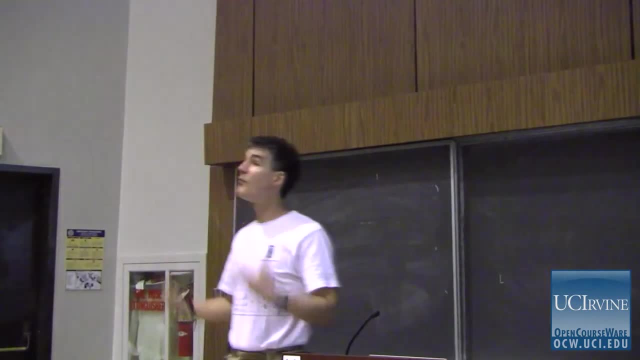 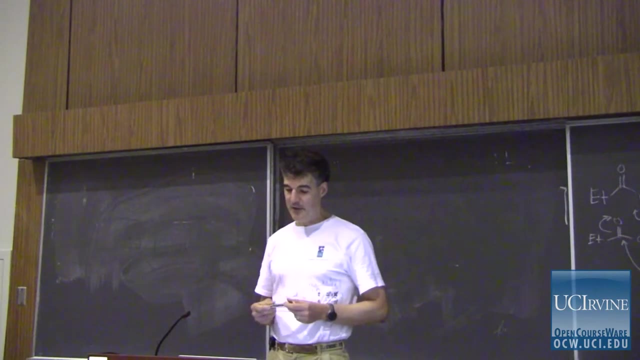 then that's very awkward and that takes more energy than doing it in a more natural way. now you can use Mathematica. if you take Chem 5, which I recommend that you do- you'll learn how to use it and it's really unbelievably good software, in my opinion. 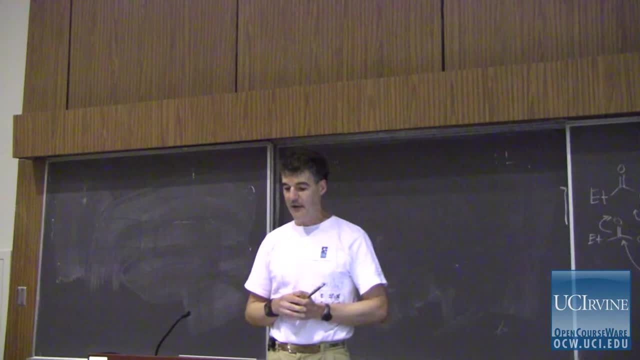 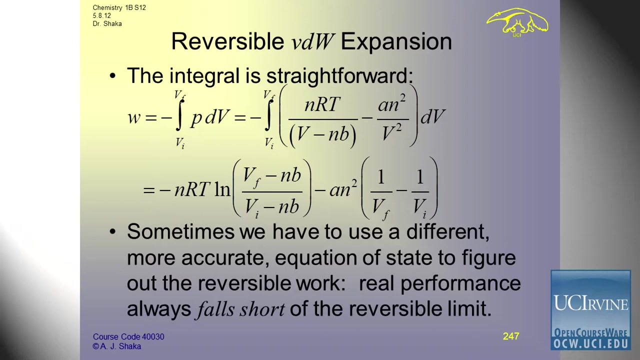 ok, I went to integralscom and I handed it this, and this is what it did: I get a term that's like the other term, but now it has this subtracted volume off for the NB. and then I get an additional term, which is due to the attractive part. 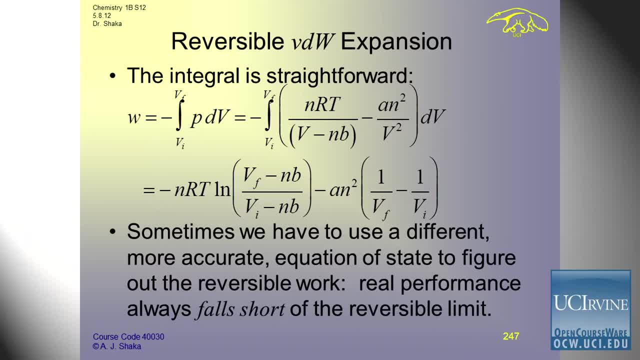 which has a different form, and that would be the most work I could expect to get out of van der Waals gas. sometimes we have to use a different, much more accurate equation of state to figure out the reversible work, especially if it's at really high temperature. 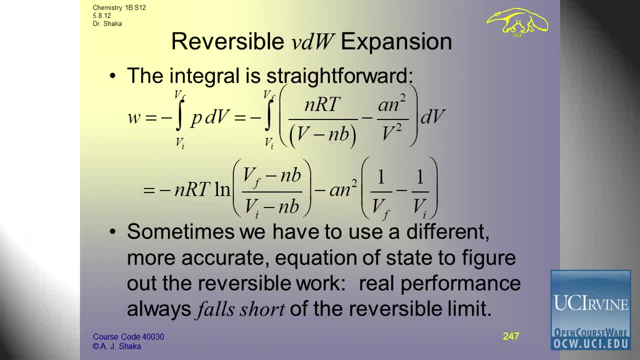 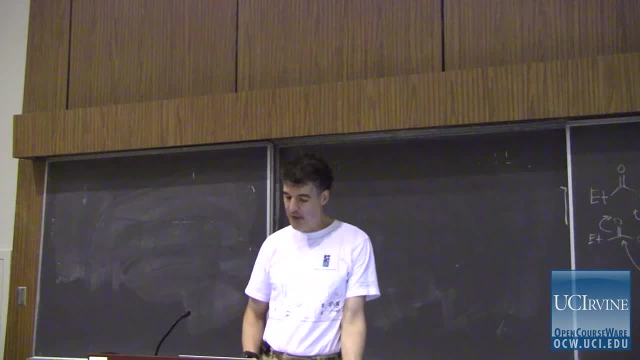 and pressure. you just have to look things up if you're really doing important work. you just become familiar with the steam tables and you calculate what you can possibly get and whatever you calculate for reversible, when you actually make a machine to try to get that work, it's going to be less than 100% efficient. 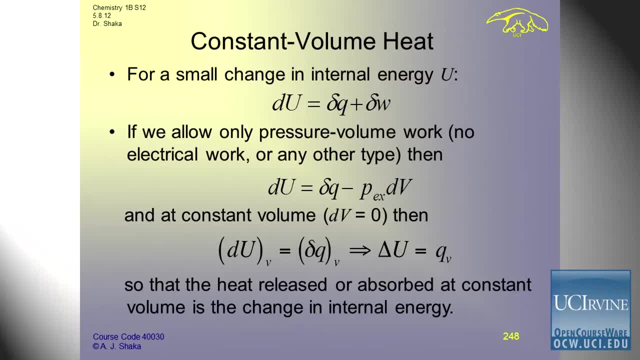 ok, if we make a small change in internal energy U and we can write a small change and make this a little delta. if you find the D intimidating, same thing- and I use a funny Greek delta here, because these are not really things you can integrate, because those things 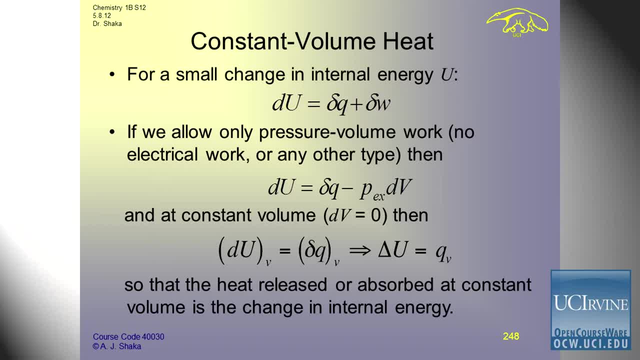 don't correspond to an area under a curve. if I have something that corresponds to an area under a curve, then if I go to here and then I go back and then I go to here, I get the same area under the curve, because it's a good thing. 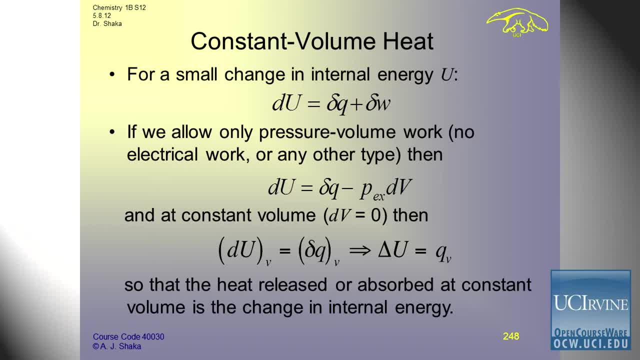 that totals up, if I have something that doesn't correspond to an area under a curve- it's like, for example, having a spiral, if I have a two dimensional surface and if I have a spiral. so I go around and I come back and I'm up above. 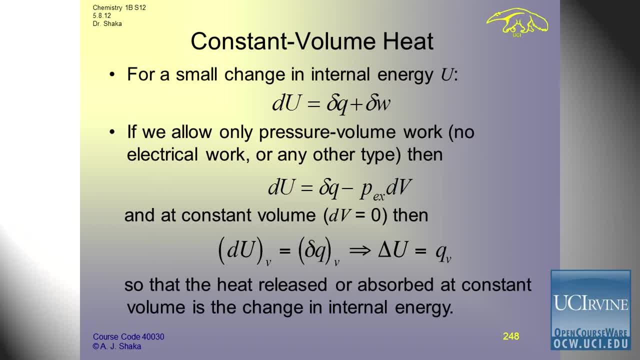 where I was, and then I go around again and then I'm up here, then I can't tell that. that doesn't correspond to any area under a curve and that's like friction. if I keep rubbing something, it depends not where my hand starts and stops, but it depends how many times. 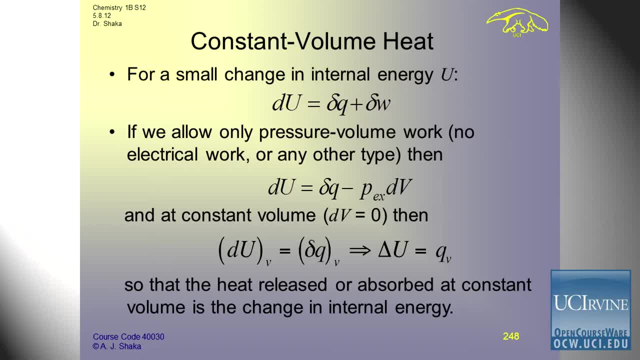 I rub the thing- how much energy gets dissipated as friction. so friction, which is heat alone, is not something that's conserved. if you minimize friction with oil, you get better work out than if you have high friction. then you just waste a ton of energy turning work into heat. 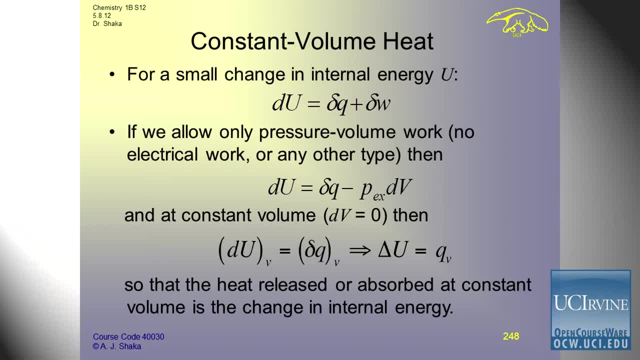 if we only do pressure volume work, we know what the work is. that's just the external pressure times, whatever the change in volume was. and if we say, gee, what if we do it at constant volume? well, constant volume means that dv is zero and that means that the change in internal energy 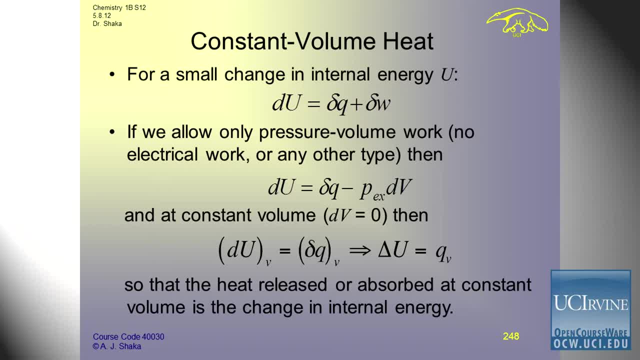 at constant volume is just the change in heat at constant volume, and if I integrate this becomes a delta, u and this just becomes q: the amount of heat added or subtracted at constant volume. and this tells us that if we keep something at constant volume and then we add or subtract heat, 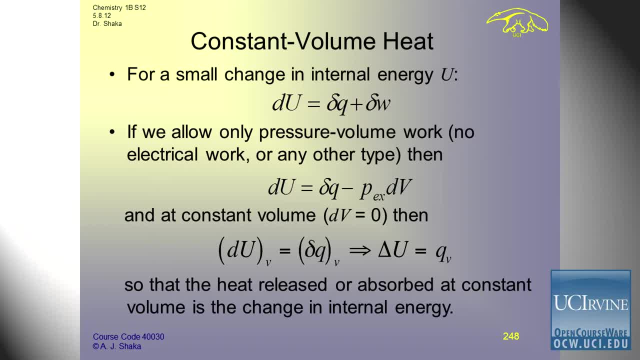 that's just going to change the internal energy of our system. constant volume is another idealization because most things when you heat them they expand very hard in the lab to keep things at constant volume. so this is kind of interesting theoretically but practically not that useful since it's very hard. 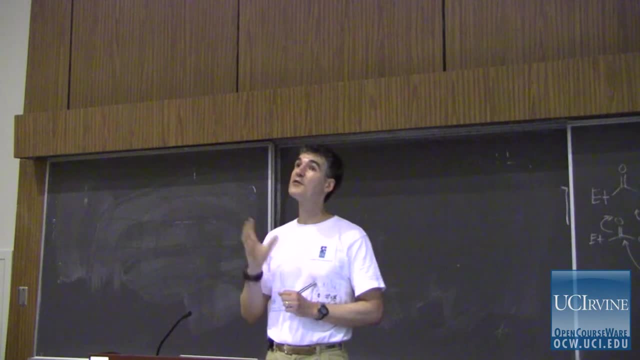 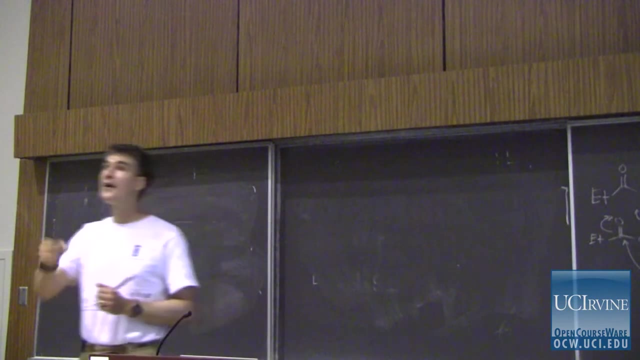 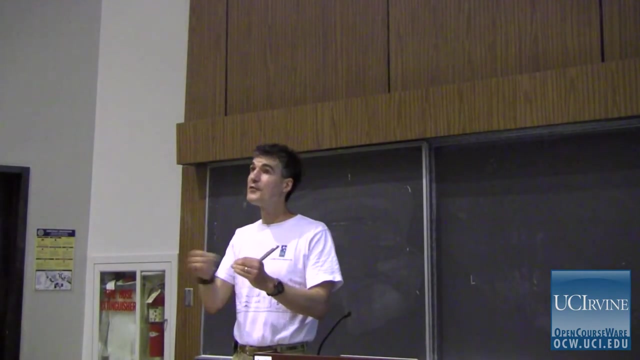 to do the experiment. on the other hand, every chemistry reaction we do is at constant pressure because we usually have an Erlenmeyer, we're swirling it around, it's in the lab at one atmosphere of pressure and so that we do often and we're very much interested. 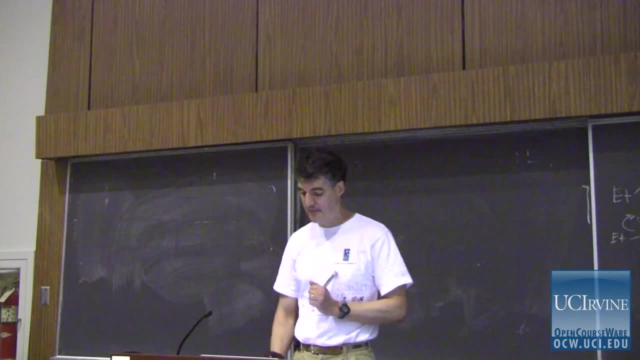 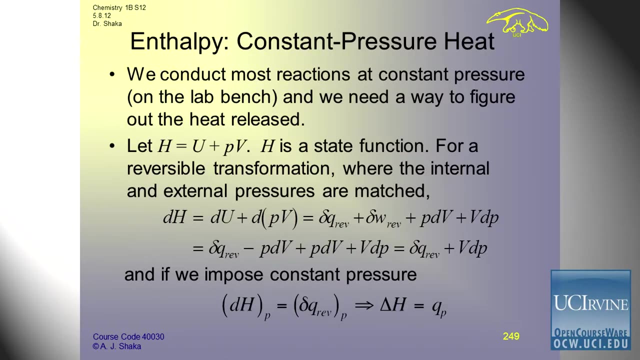 in the heat at constant pressure, and that's called the enthalpy. we conduct most reactions on the bench at constant pressure and we need to figure out how to calculate the heat released. we need to invent a state function so that we can keep track of it. 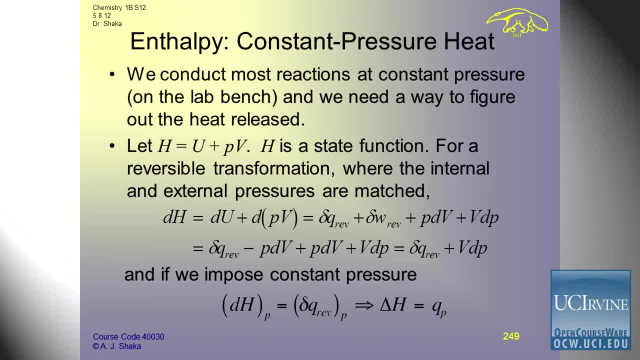 no matter how we did the reaction, because we don't know what the reaction is. and the trick is we make a new function. U is a state function and PV is a state function, because if we specify the state, we specify P and B. therefore, H is a state function. 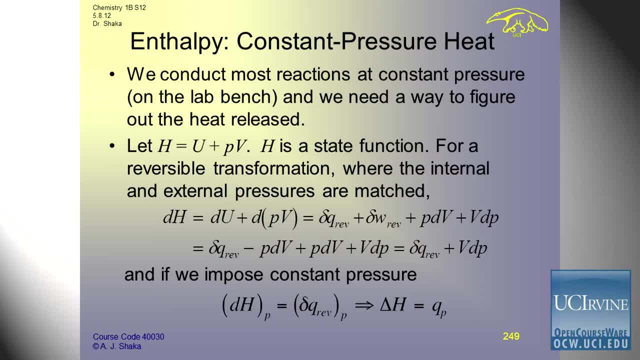 and then we take H and we just do a little calculus, we take its derivative. if you don't like just DH, you can always say DH, DX, if you've done that, and then at the end you can get rid of all the DX's but the derivative of H. 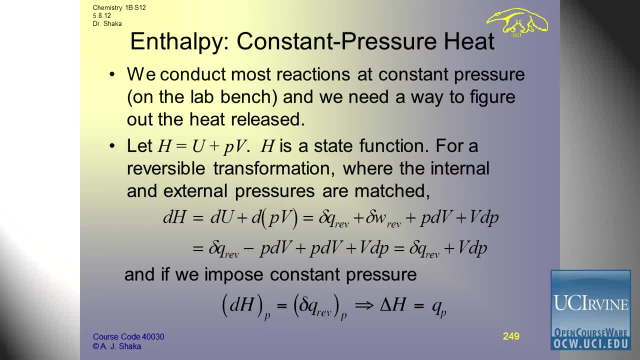 is the derivative of U plus the derivative of the product U is this, if it's reversible, and the derivative of the product of P times V is the first times, the derivative of the second plus the second times the derivative of the first and then the reversible work. 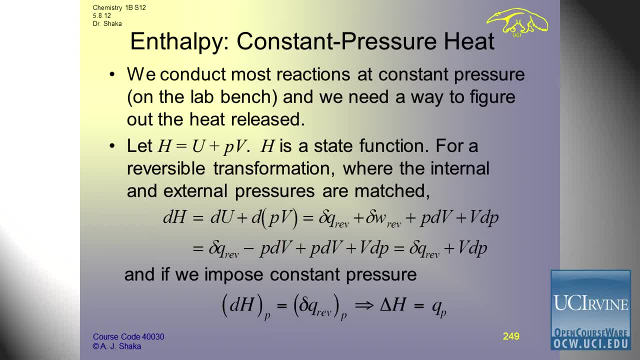 here is minus PDV. so beautifully PDV goes away and we have the reversible heat and VDP. and then if we say, hey, we don't let P change, then what we find is that the change in this state function we made up, which we're going to call 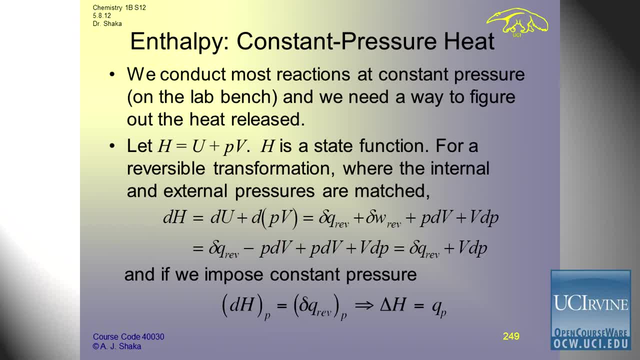 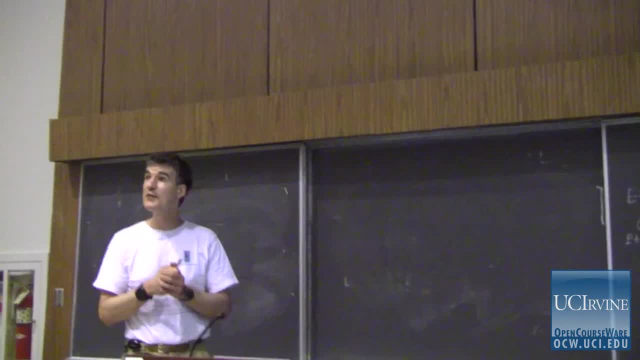 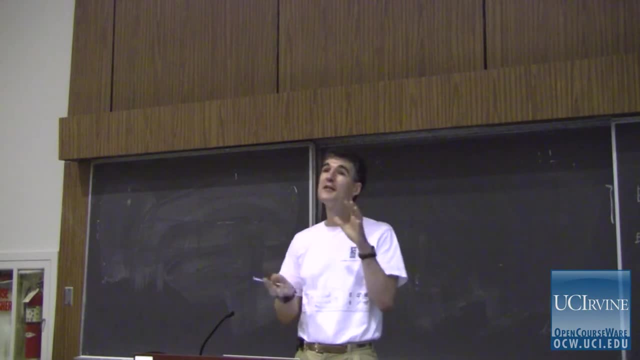 enthalpy is the heat released or absorbed at constant pressure, and that's very important because that's how we do chemistry reactions. we usually do them at constant pressure. you have to be a little bit careful when you do these calculations in a car cylinder. it's not constant pressure. 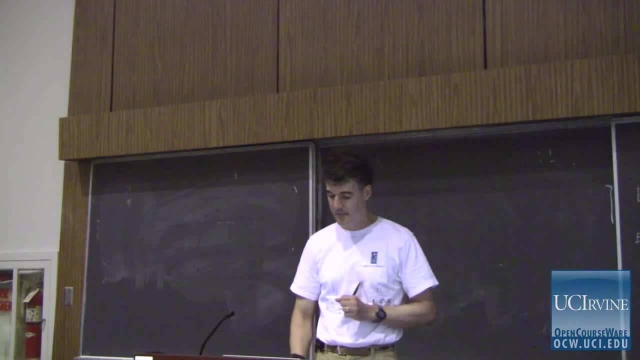 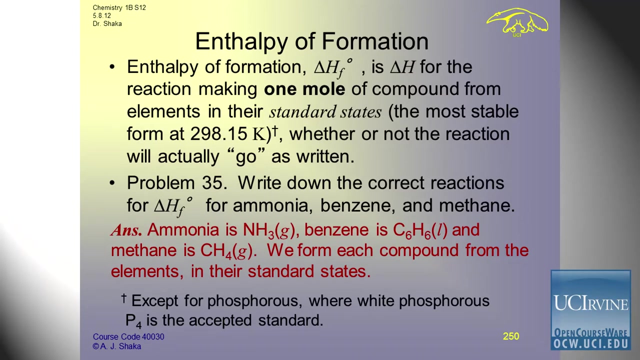 because you're pushing down and then it's expanding and so forth. calculation is much more difficult than this, but anyway this gives us an idea. if we want to figure out what heat will be released or absorbed at constant pressure, we could either do any possible chemical reaction. 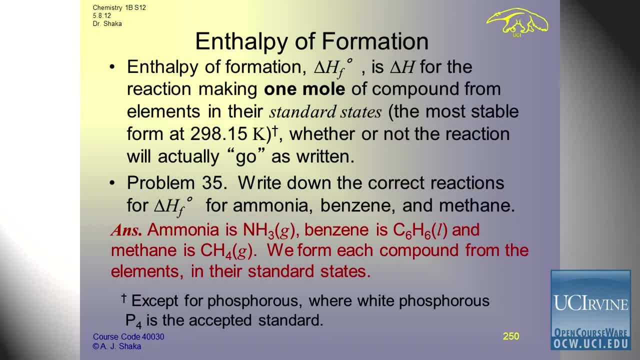 or we could kind of have a system where we have certain numbers that we know and then we add and subtract things. because it's a state function, we don't have to know how it happened. we add and subtract things and then we get what we want and the most important. 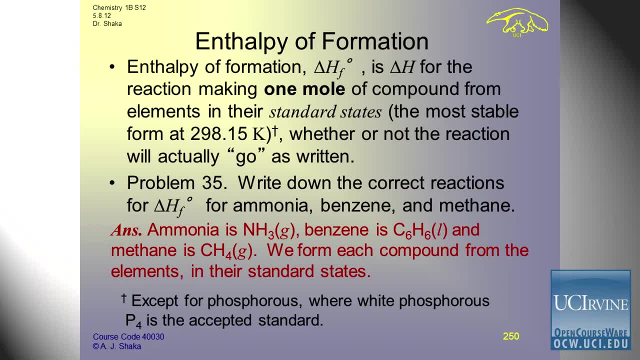 invention along these lines is called the enthalpy of formation. it's the heat absorbed or released at constant pressure when you make one mole of a compound from elements in their standard states, which the standard state is usually at 298.15 Kelvin, but it's always at 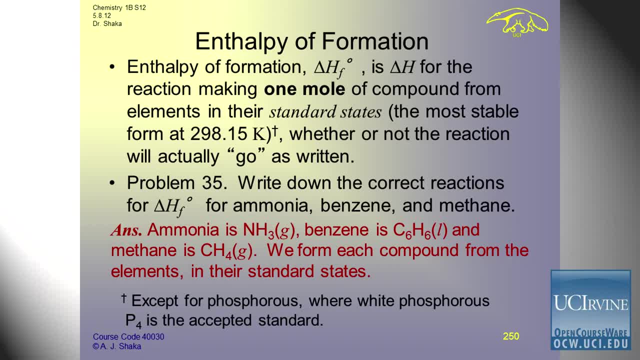 one atmosphere or one bar. they've probably updated it now. pressure: it's the most stable form of the element at one atmosphere pressure and usually 298, or sometimes they'll list another temperature and then that's what the standard state is at that temperature, except for phosphorus. 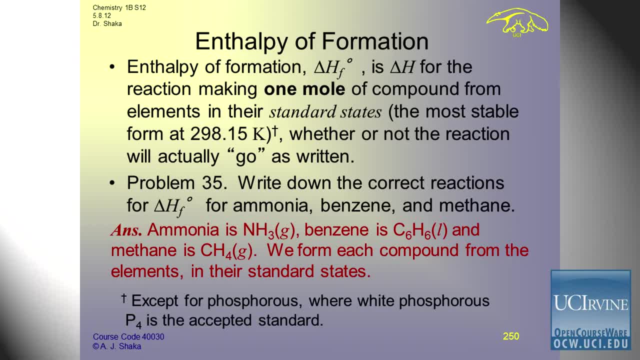 where white phosphorus is the accepted standard, even though that's not the most stable form. ok, let's do a problem: write down the correct reactions that refer to the enthalpy of formation for ammonia, benzene and methane. ok, now we have to write some pretty improbable reactions. 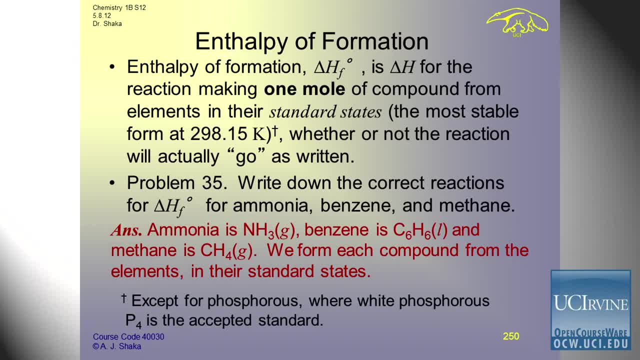 but we don't care whether these reactions will go or whether they can be carried out in our lifetime. now we first have to know what these trivial names mean. ammonia is NH3, benzene is C6H6, which is a liquid, and methane is CH4 gas. 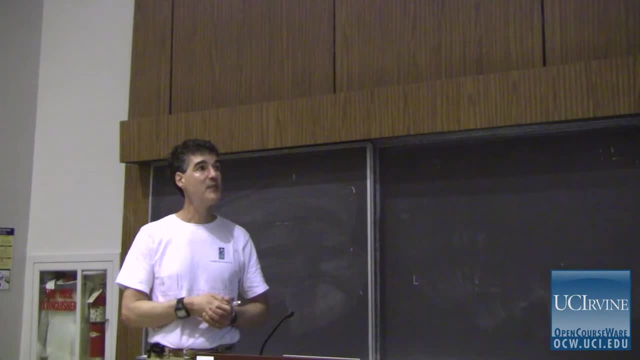 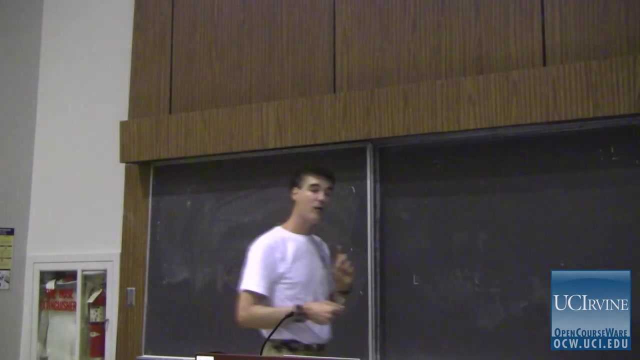 we have to form each compound from the elements in their standard states and we have to balance the equation, using fractions if necessary, so that we get one mole of compound. when they say the enthalpy of formation is blah, blah, blah- kilojoules per mole. 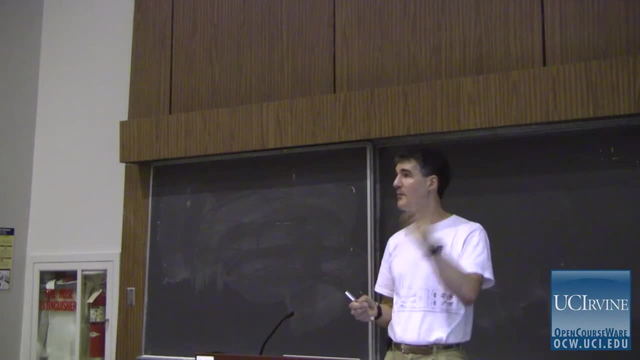 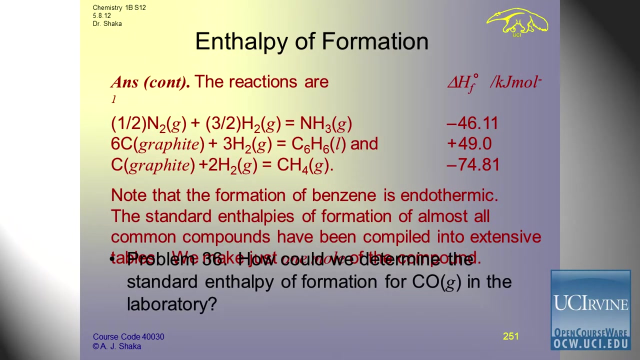 it's per mole of the compound, not per mole of the reactant or something else. and so here they are and I look them up: if I take one half N2 gas, then I get one nitrogen. if I take three halves H2 gas, I get three hydrogens. 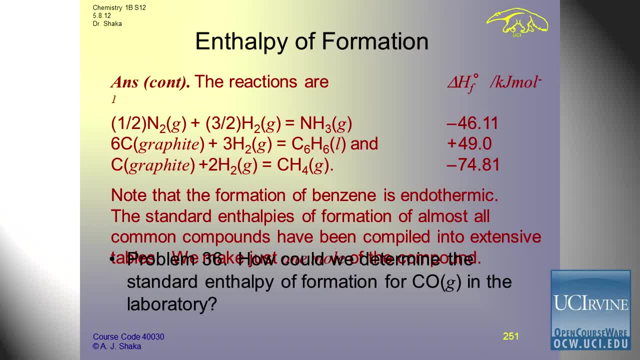 then I can take these two elements and I can make ammonia and I can actually do this. that's done on the millions of ton scale and the enthalpy of formation. it's exothermic. it's minus 46.11 kilojoules per mole. 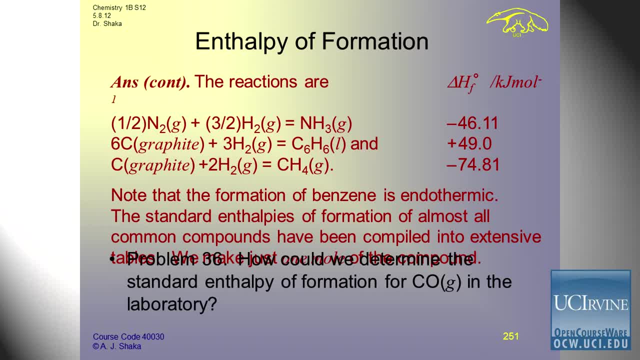 of ammonia for benzene, if I take six carbon atoms as graphite- that's the standard form, plus three molecules of molecular hydrogen and I get one mole of C6H6 liquid, and it's plus 49 kilojoules per mole. and if I make methane, 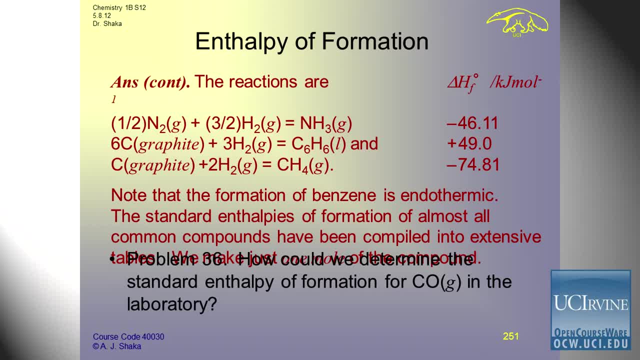 from graphite and hydrogen. this reaction, I certainly wouldn't want to wait around for it to happen. it's minus 74.81 kilojoules per mole and it's kind of interesting that the enthalpy of formation of benzene is endothermic. 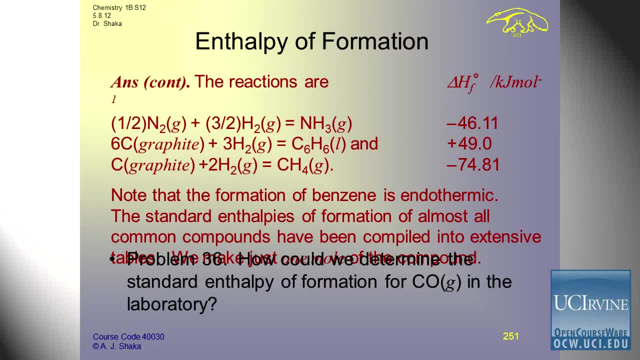 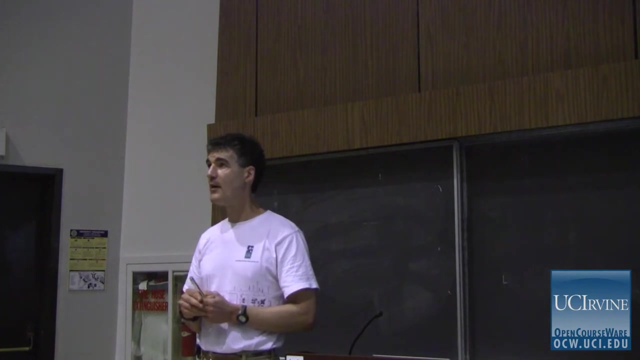 and you'll learn more about that in organic chemistry. benzene is kind of a special case in many ways. okay, let's try to figure out how we could determine in the laboratory the standard enthalpy of formation of carbon monoxide. carbon monoxide is poisonous. 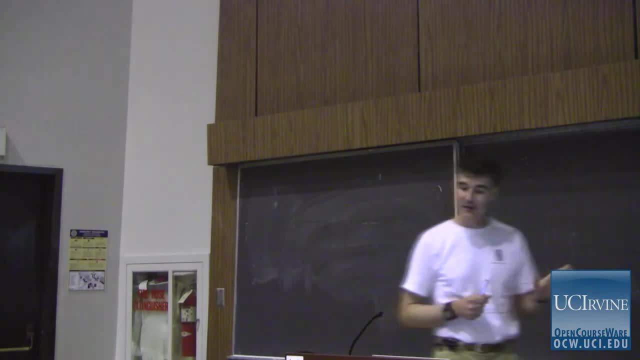 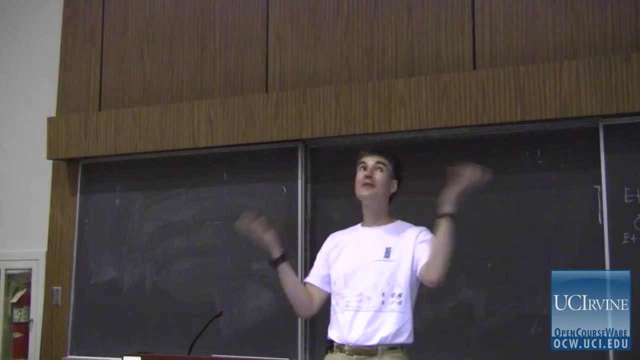 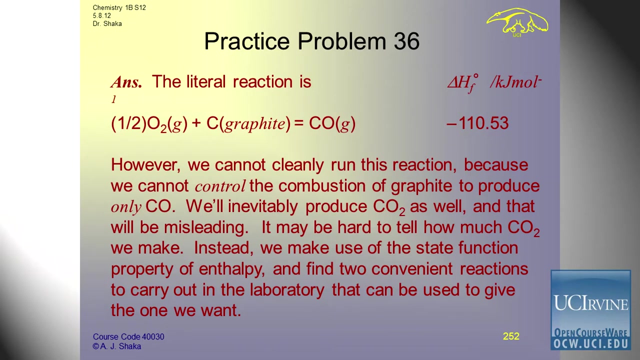 and it's a gas. chemists tend not to like to deal with poisonous gases because gases have a bad habit of getting away from you and once they get out into the atmosphere they're very hard to get back the genie back into the bottle by far. but we have to deal with gases. sometimes. here's the literal reaction. if we just look it up, we take one half of a molecular oxygen, plus C as graph, carbon as graphite, we get one mole of carbon monoxide, and it's exothermic to the tune of minus 110.53 kilojoules. 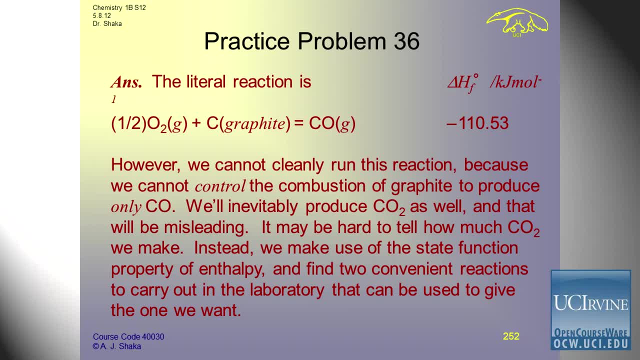 per mole. however, we can't do this reaction in the lab because we can't ensure that when we burn the carbon, we only get carbon monoxide, because usually when you burn carbon you get carbon dioxide. and how are we going to stop it adding two oxygens? it does that very easily. if it didn't, we'd get carbon monoxide poisoning, because every time we lit a fire we'd get tons of carbon monoxide coming up and it would kill us. so usually it burns to give carbon dioxide and therefore we can't literally do this reaction. 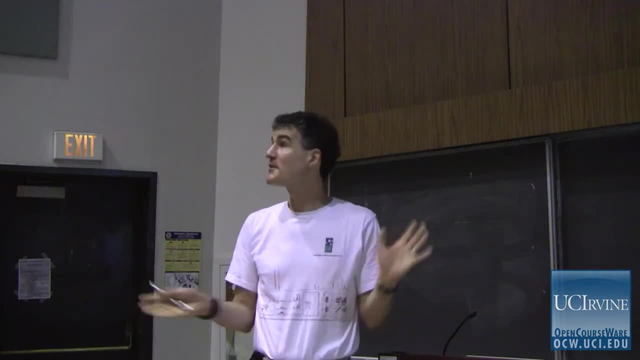 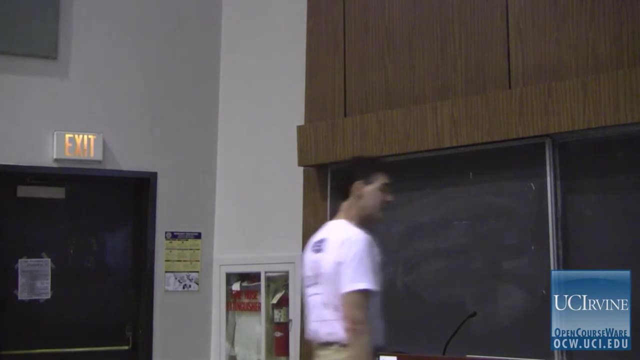 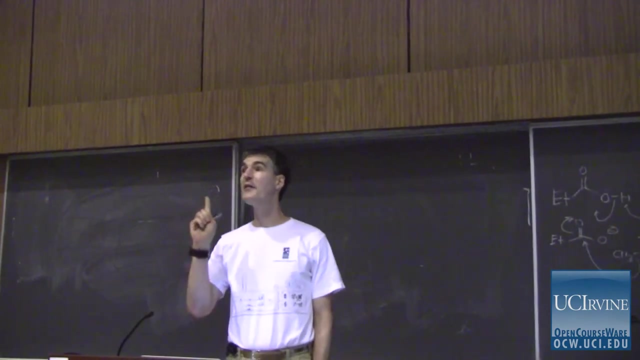 we could do this reaction in the lab, but we can't get it to go to this product. we're stuffed, we get carbon dioxide. so what we do instead is we say, hey, whatever it is doesn't depend on how we made the mole of carbon monoxide. 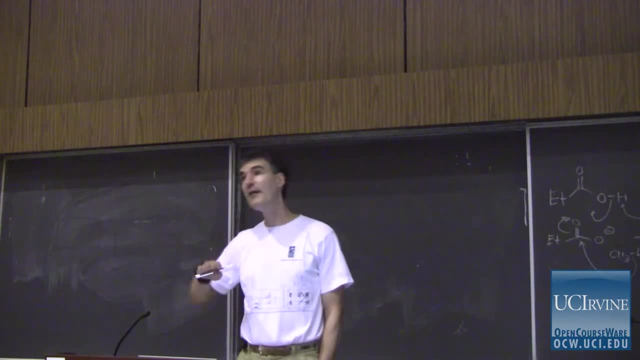 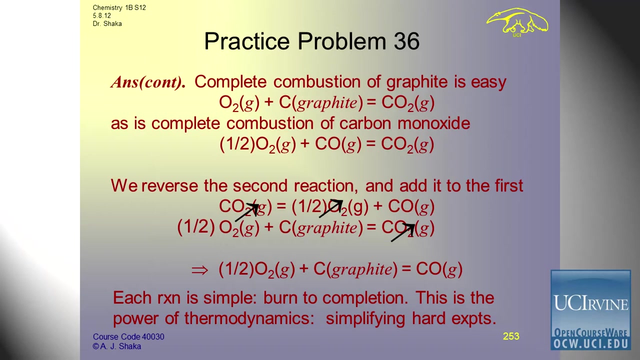 because enthalpy is a state function. we have to figure out a way to go around it so that we actually have two easy experiments. and here are the two easy experiments. first of all, we burn graphite completely. it's easy to burn something completely because you keep burning and burning. 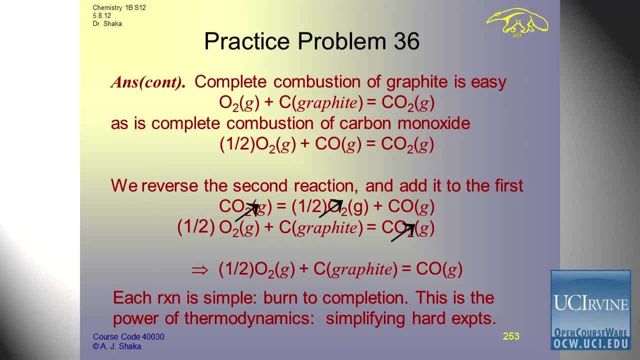 until it's all burned up, that we can do and that we can measure the heat and get CO2, and then we can get a canister of carbon monoxide that somebody's purified and we can burn that completely as well. so now we have two reactions. 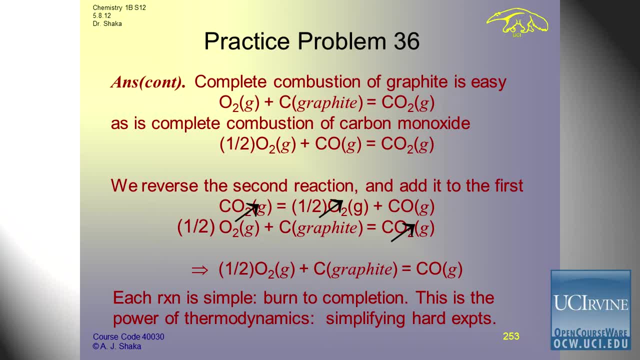 we burn graphite to get carbon dioxide and we burn carbon monoxide to get carbon dioxide, and then all we have to do is add and subtract, because we can measure the heat of both of these. no problem if we reverse the second reaction and add it to the first. 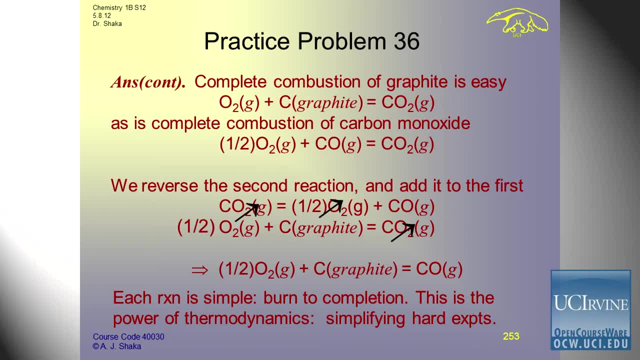 we get this situation and then we can cancel out things that we don't need and we get the reaction we want. and therefore, if we just take this one here, measure its heat, we measure this one and we reverse it, we'll get what we want and each reaction. 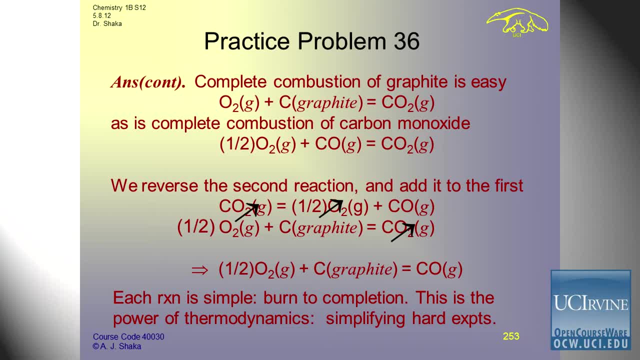 is pretty simple because we just burn it to completion, and this really is the power of thermodynamics is that you can get something. you can get a number for something that you want to get. that is extremely difficult to actually measure accurately in the laboratory by measuring two things. 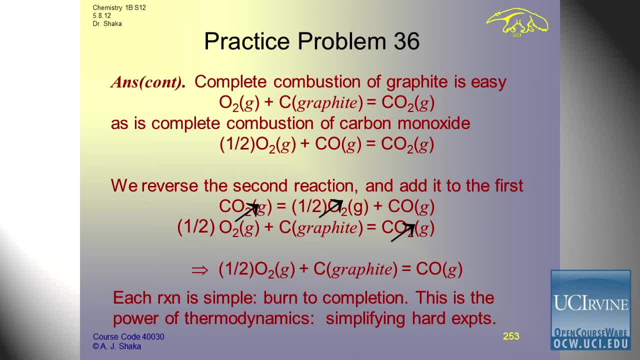 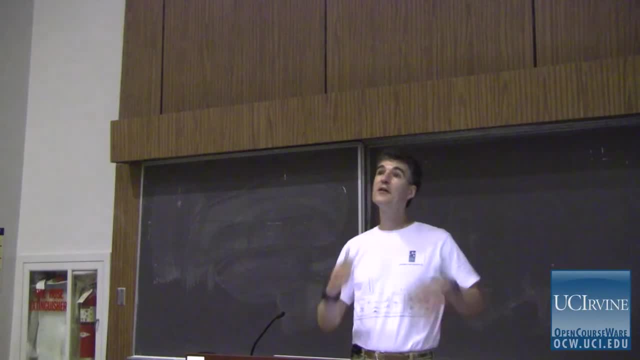 that are easy to measure accurately and then using the power of the state function to tell you the answer you want to get. and what that means, then, is that, if you look at the table of all these enthalpies of formation, they all look like random numbers. 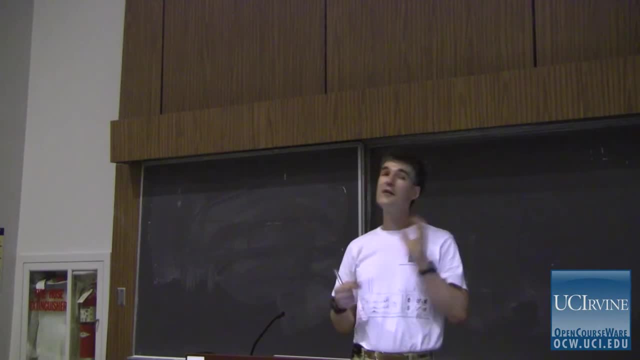 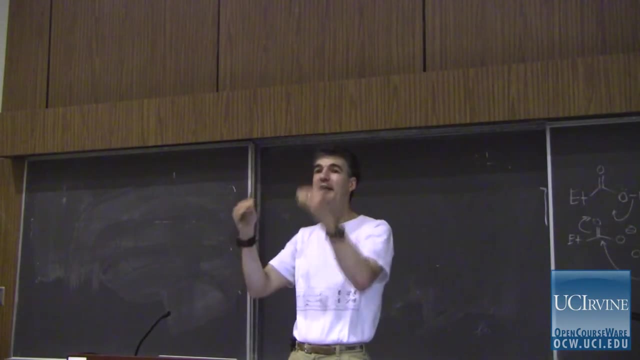 at first, but in fact they're not, because they all have to fit together like pieces of a puzzle, because if I add and subtract this to that, it has to be this number over here that's also in the table or something's wrong, so they all have to be. 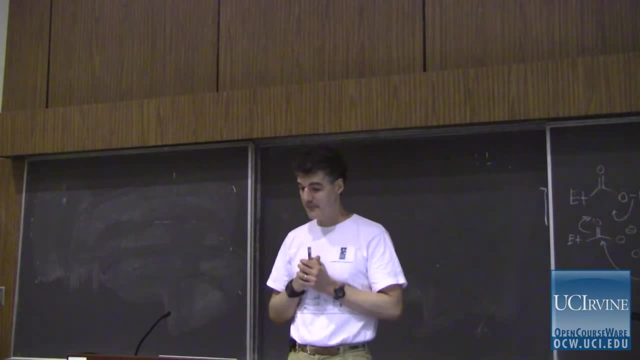 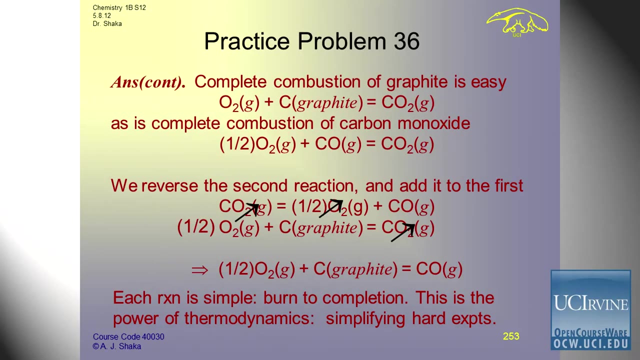 yes, well, because here's how they cancel out initially. initially, to get this CO2. here I have a whole O2 and I have half an O2 here. so when I cancel the half, I put a half here and the CO2 goes away with the CO2. 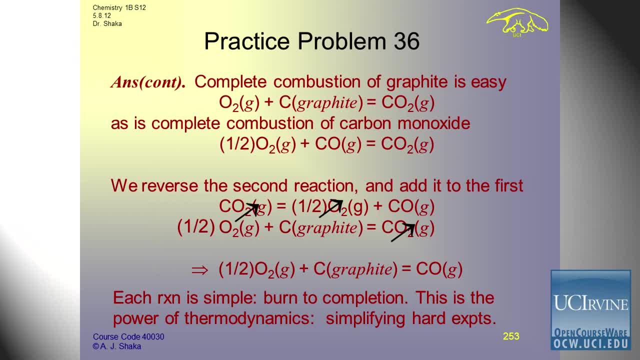 so it's out of our hair and so that's where I put the half in there. that's how it disappeared, okay, and then the only things left are half an O2 and C graphite, and then the only thing left on this side is CO. everything else is gone. 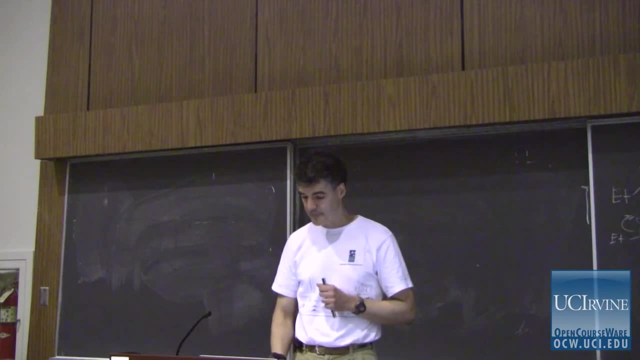 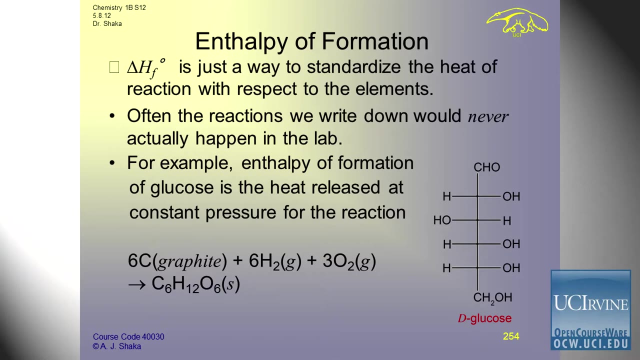 this is the one, then, that I want. okay, the enthalpy of formation is just a way to standardize the heat reaction with respect to the elements, but often times, the reactions that we would write down are just never going to actually happen in the lab, for example. 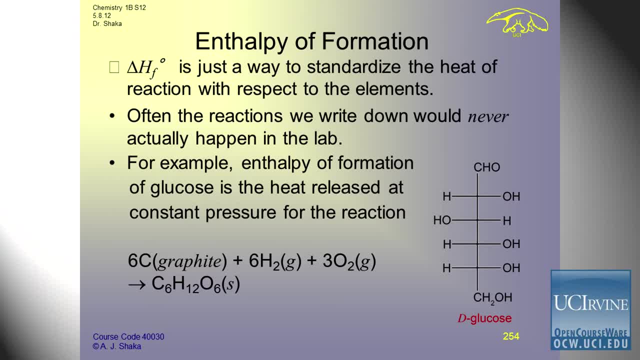 you can look up the enthalpy of formation of glucose. here's glucose in the open form circulating in your blood at about 80 milligrams per deciliter, or much higher than that if your pancreas has given up the ghost because you've eaten so much sugar. glucose is highly regulated, like sodium, in your blood. your body does not want a ton of glucose circulating in your blood. glucose is fuel for energy but much like I fuel a car, I put in gasoline in the tank and then if I say, gee, I want more energy. 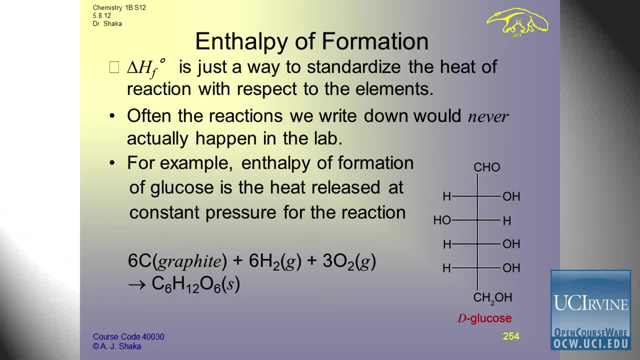 so I think I'll start putting gasoline in the passenger compartment and all over the roof and everywhere else. the car doesn't work well. the reaction for glucose literally is to take graphite, hydrogen and oxygen and get this, and then you can. you can never carry this out. 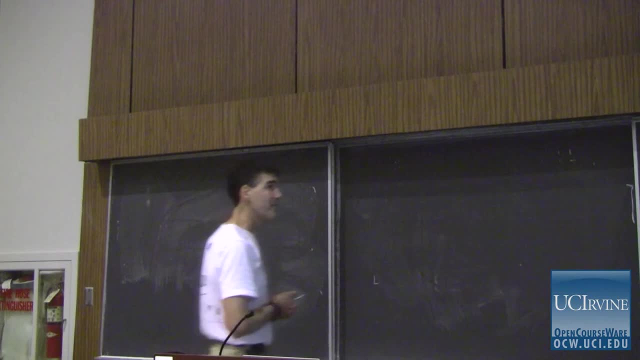 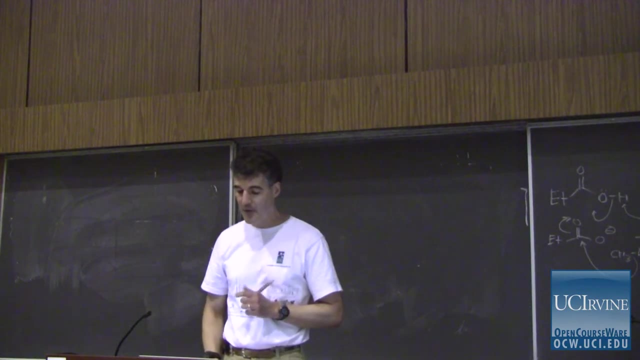 in the lab, but you can write it down and it has a number in the table for the enthalpy of formation. it doesn't matter whether you can actually carry the reaction out from the elements. often you can, once we know the enthalpy of formation. 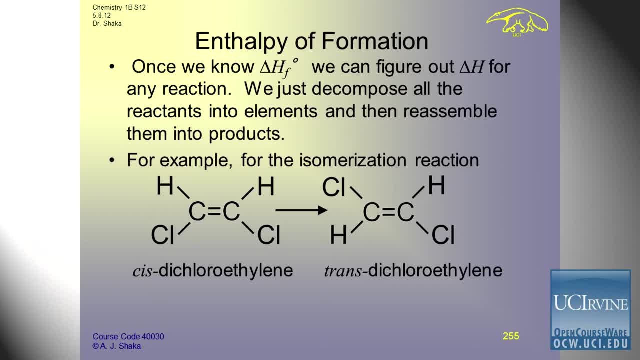 we can figure out delta H for any reaction, because we just decompose all the reactants into the elements and then just reassemble the elements into the new products and we've got numbers for every step. if we want to react glucose with something, we first take glucose. 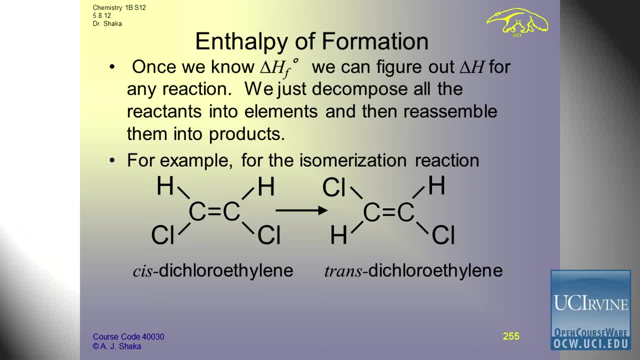 and we turn it into carbon, as graphite hydrogen, as molecular hydrogen oxygen, and then we take those and we assemble them back together into some other product and that's the enthalpy for that reaction. for example, here's an isomerization reaction: cis-dichloroethylene. 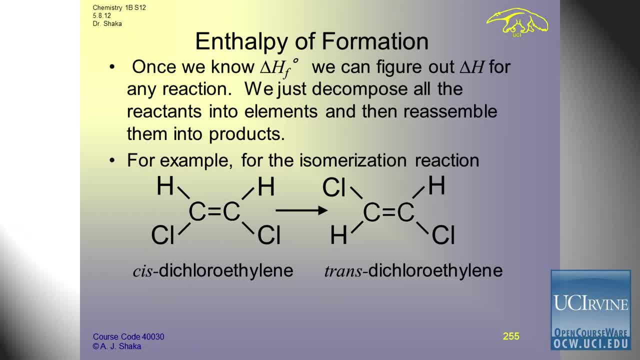 the chlorines are on the same side. once you've got a double bond, it can't rotate anymore just like a flat plane sitting there floating around. you've got a single bond, about 10 to the 13 times per second, which is pretty fast. these don't. 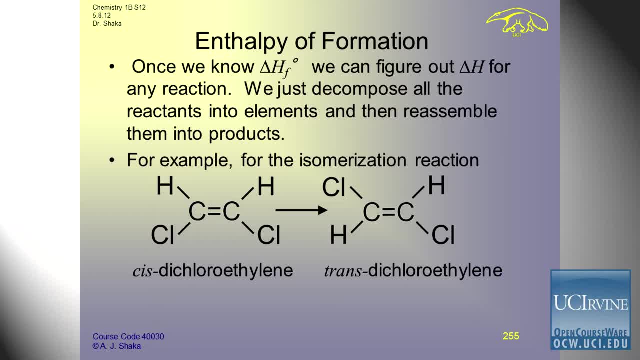 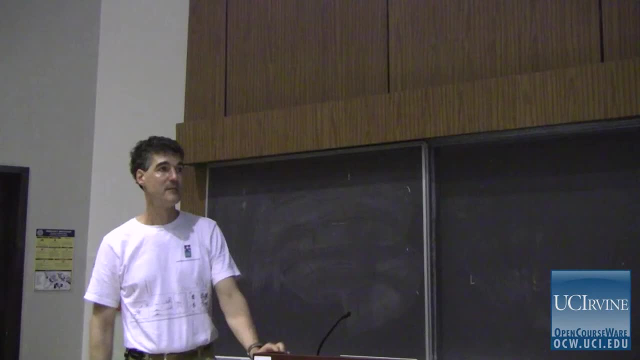 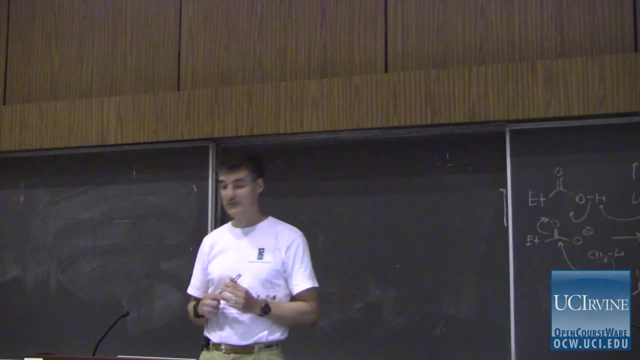 and therefore these two are different. when the chlorines are across, this has a different dipole moment than this. this has a different boiling point than this. this has a different human toxicity to your liver than this and so forth on the same side, and trans is across. 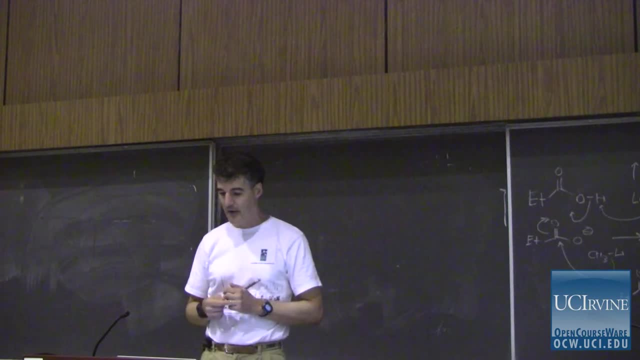 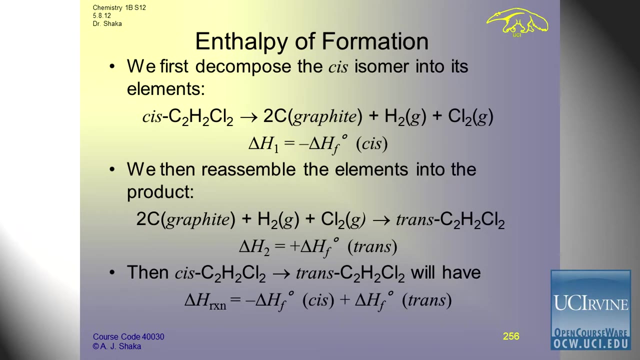 across the tracks. well, let's first decompose the cis-isomer into the elements we make- graphite, hydrogen and chlorine- and the energy to do this, the heat will be minus. delta H of formation is starting with these three and getting this. so if I reverse the reaction, 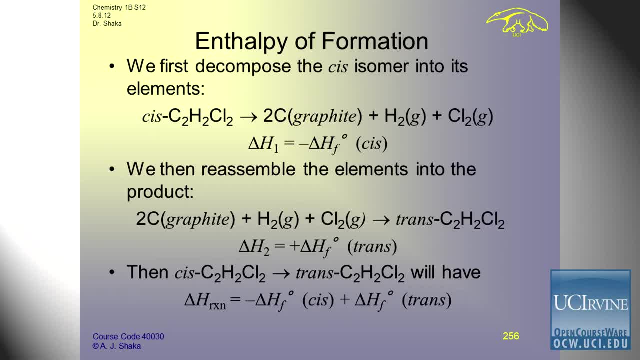 I reverse the sign of delta H, because I'm reversing the products and the reactants, and then I just take those same three and I reassemble them into the trans and I look up delta H of formation for the trans in the table and then delta H for that reaction. 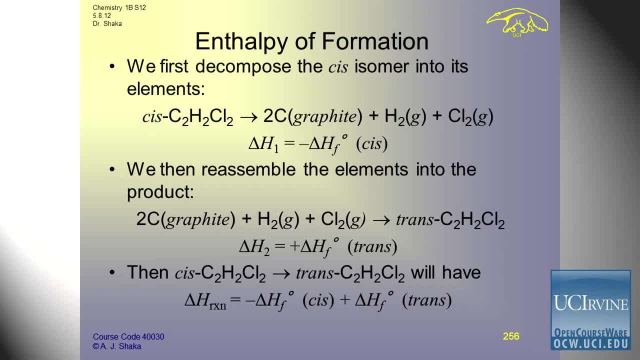 which I can't do. I can't go in there with a pair of tweezers and just go like this to every molecule. I don't have that kind of control. but I can still figure out what delta H for this hypothetical reaction would be from turning cis into trans. 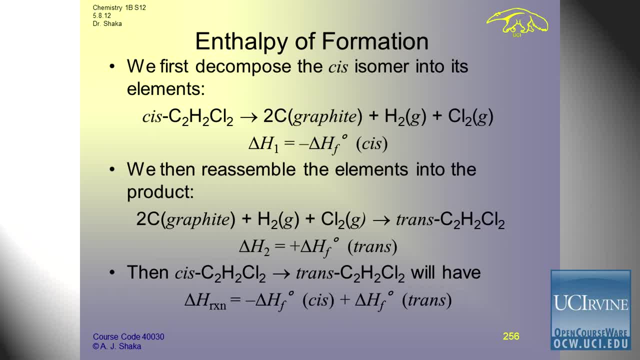 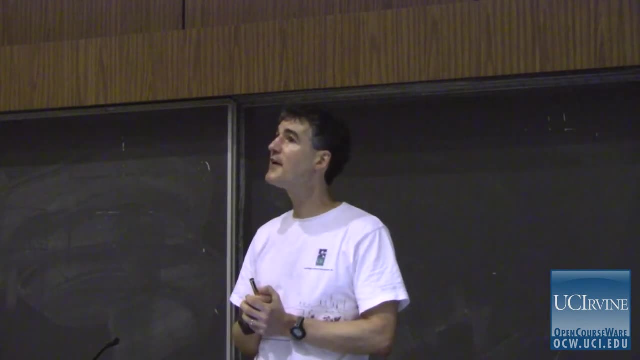 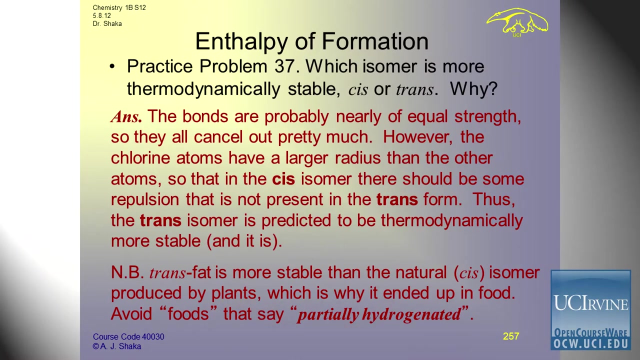 it's minus delta H of formation for cis, plus delta H of formation for trans, and then I can figure out: is that exothermic or endothermic? will that release heat when I turn cis to trans, or will it absorb heat when I turn cis to trans? 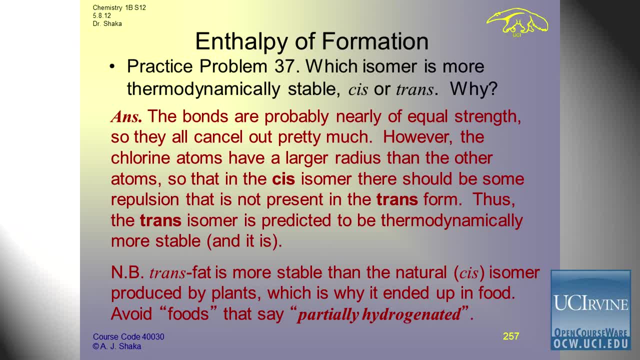 okay, which isomer do you think, without knowing anything? I realize you don't know anything. yes, could you go back on the slides at this moment I will post the slides so you can look at them. which one do you think is more stable, cis or trans? who's lower down? 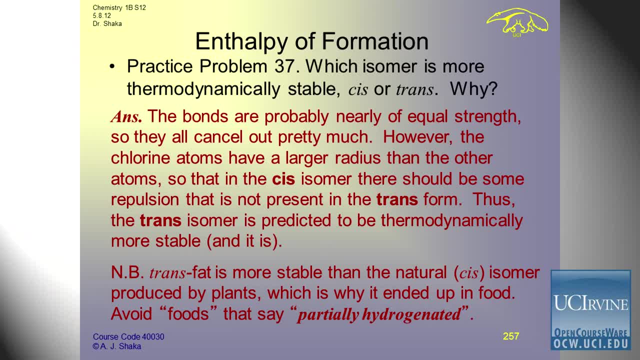 and five, because the more stable one is the one we'll tend to get if one of them is valuable and the other one's not, and the one that's not valuable is more stable. I'm in trouble because I'm going to get a ton of stuff. 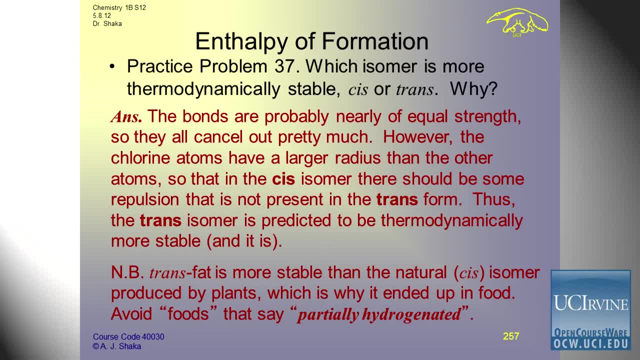 I don't want. it can be quite important to know. well, if you look at them, they all have the same number of atoms stuck together because they are isomers. that's essentially what isomers are, and so the bonds are probably nearly of equal strength, and I would guess 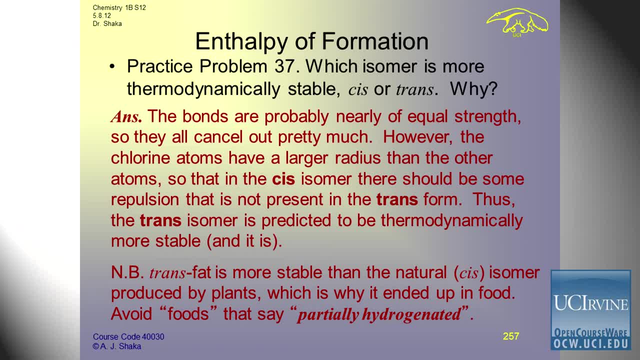 they cancel out pretty much. but the big chlorine atoms- and when we just draw these, these letters, we aren't really drawing how big these are- the chlorine atoms are closer together on the cis because they are right across, so they are like two big balloons annoying each other. 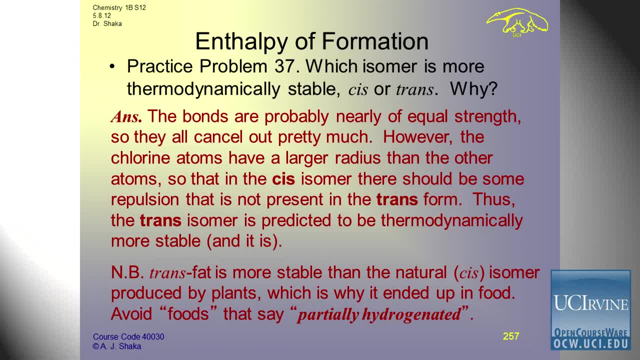 hey, get out of here, hey, get out of here, and they prefer to have more room. and so if I rotate this one over to the trans, where they are further apart, that's going to be more stable, and that's in fact true, and unfortunately, trans fat is more stable. 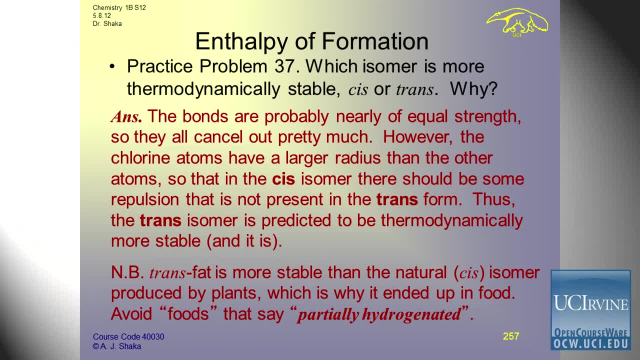 than the natural fat, which is the cis isomer which is produced by plants. if you look at fatty acids that are unsaturated, that means they have a double bond. plants always produce things where the carbon chain comes out on the same side of the double bond, and they tend to be oils. 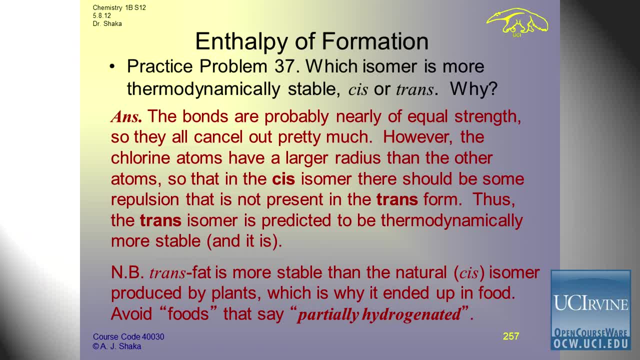 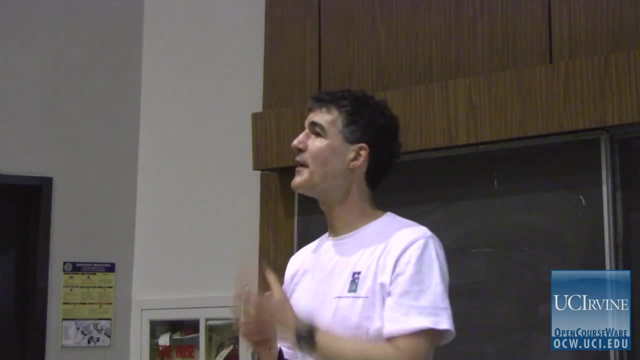 like corn oil, soybean oil and what chemists did when there was a big worry that people were eating too much. large is. they said we will produce a fat with a double bond. it will be unsaturated and unfortunately it was the trans isomer which, interestingly enough, didn't spoil. so if you put that fat into twinkies, they would be good for months and months, because bacteria didn't like that fat either. things that bacteria don't like are not good for us, and things that kill bugs are not good to breathe, and so what happened was: 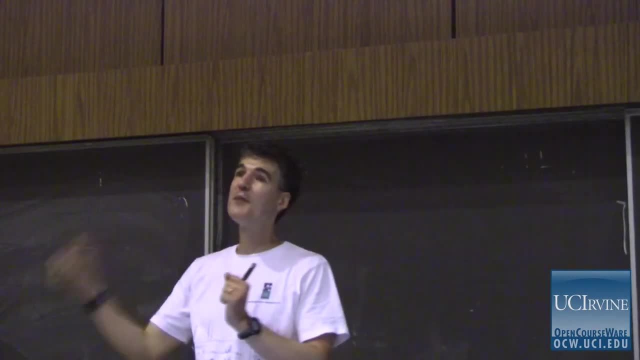 a lot of health conscious people switched from butter to margarine and ate a ton of trans fat in the 70s and 80s and then they died of a heart attack. and then the health authority said: why is this trans fat? does that promote heart disease? 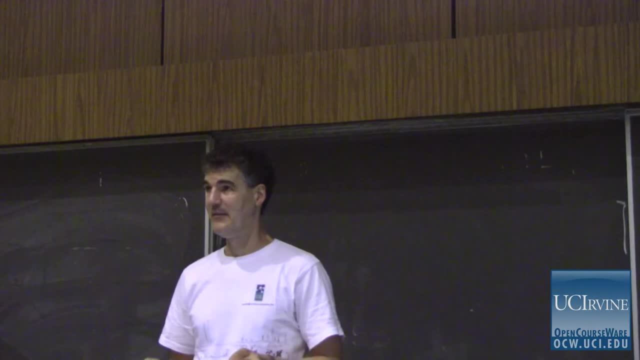 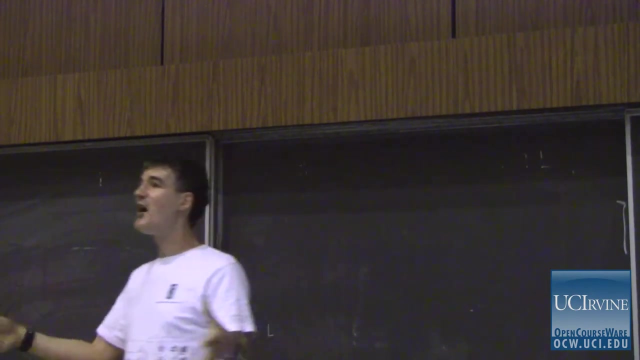 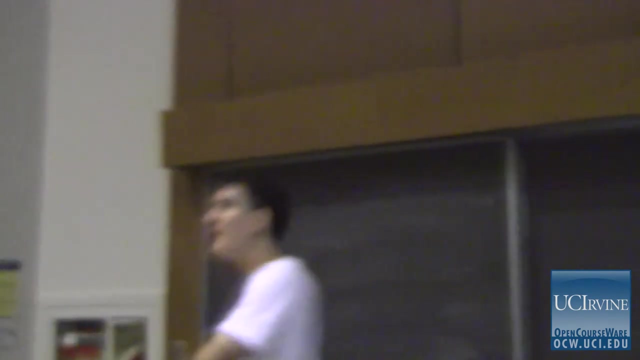 and it turns out- of course it promotes it like crazy, worse than lard, worse than just saturated fat. so it had a double bond. but in fact, because it was a cross, it would stack up. and trans fat was this vile solid material, white and just terrible, and you just throw it in. 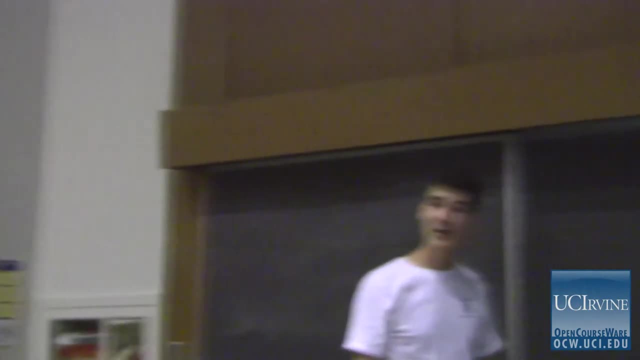 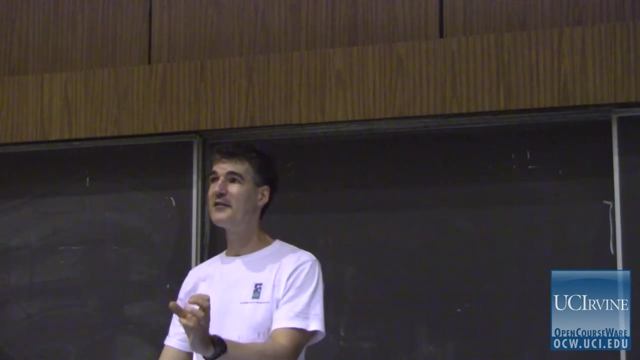 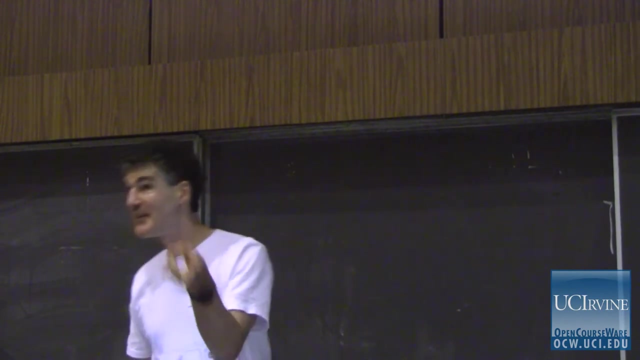 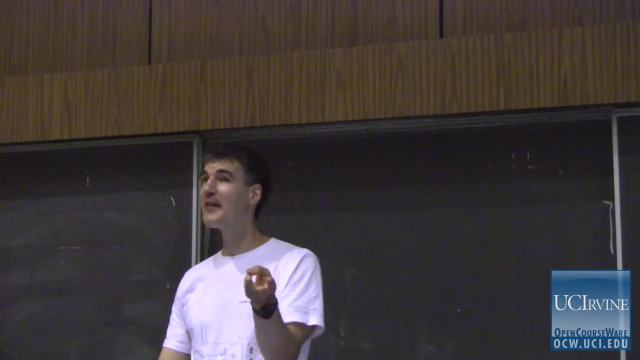 a ton of donuts or whatever with it. and then people, people tend not to eat fat on its own. I've never seen anybody take a stick of butter and just go. but if you take fat and flour and sugar, people go wild and they eat the same amount of fat. 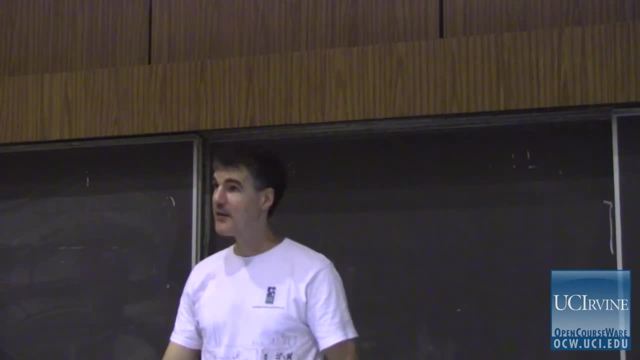 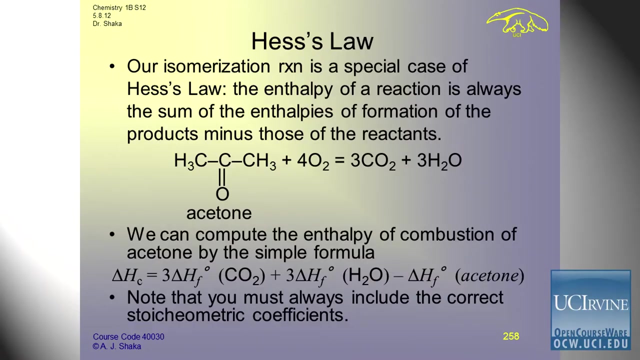 but they don't realize it, and so the rule is: if the fat is solid at room temperature, don't eat it, at least not much. if it's liquid, you're probably better off. okay, let's talk about Hess's law. it turns out our isomerization reaction. 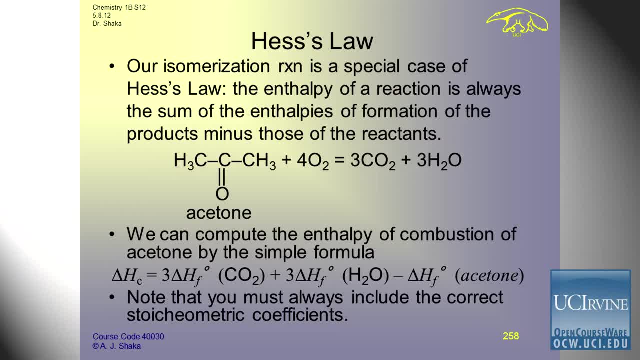 is just a special case of Hess's law. in fact, Hess's law is nothing other than the enthalpy is a state function. so the enthalpy of a reaction is always the sum of the, the enthalpies of formation of the products, minus the reactants. 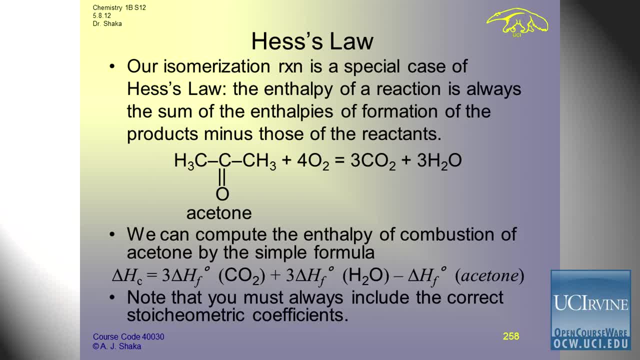 for example, if I want to figure out the combustion of acetone, here's acetone used in fingernail polish and all kinds of things. get that smell and I take acetone and I burn it. it will burn with oxygen. I'll get 3 moles of CO2. 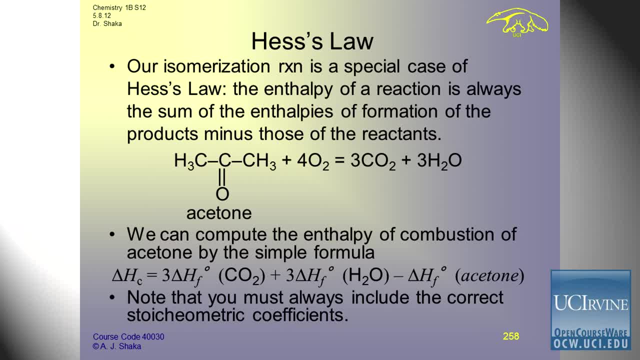 and 3 moles of H2O. then I can ask: okay, what is delta H for this reaction? and the answer is: if I know delta H of formation of all these guys- and this is an element- in its standard state is always zero. then I have these: 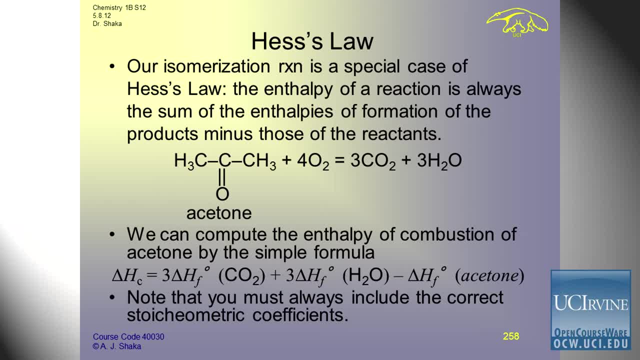 three that I have to look up in the table. it's duck soup. I just look them up and I have to multiply them by the numbers, because delta H is for one mole and I made three moles, so I'm going to get three times as much heat. 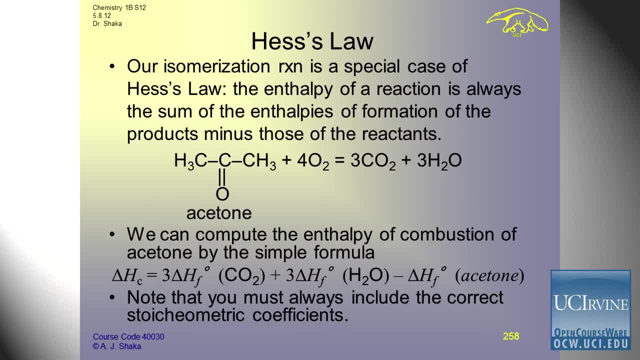 therefore the delta H, the enthalpy of combustion, is just three times whatever the enthalpy of formation of carbon dioxide is, plus three times whatever it is for water. those are the two products, minus whatever the formation is for acetone and then O2 being an element. 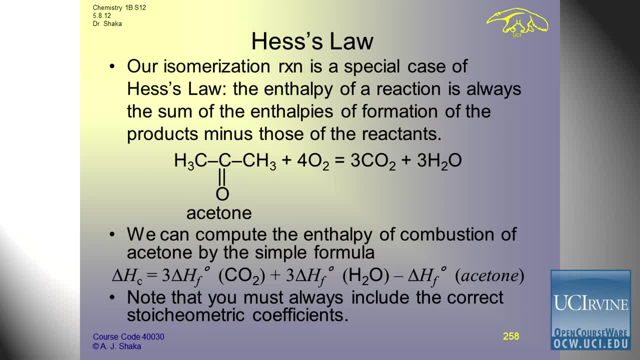 the delta H of formation is zero, so I didn't bother to put it in. but I could put in delta H of formation and put it in as zero, and that's how you have to do it. you just have to be sure that you include the threes. 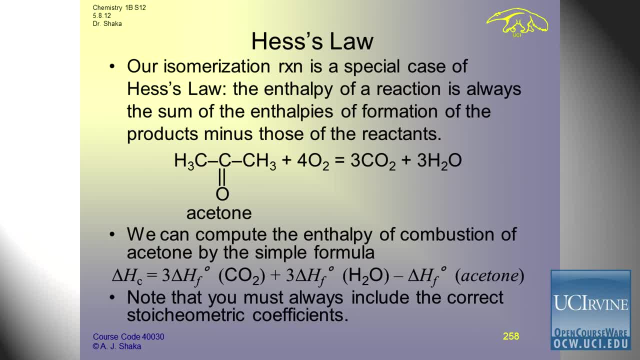 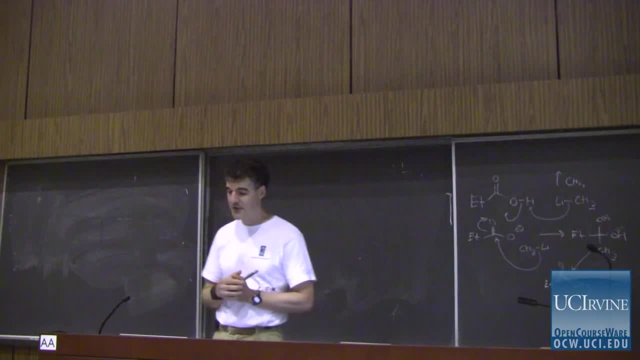 here because it is per mole and you made three moles, so it's three times as much. and that's why you have to be able to balance chemical reactions, because if you get the numbers wrong when you balance the reaction, then you get the heat wrong, then everything is wrong. 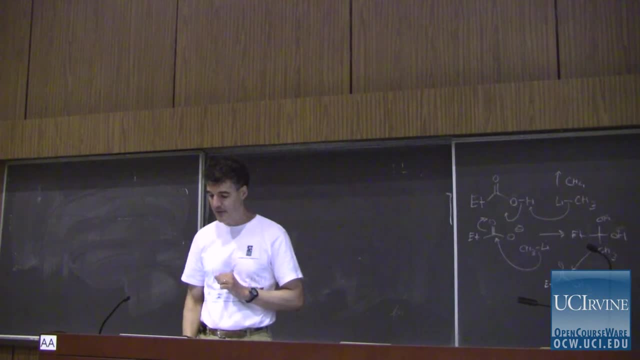 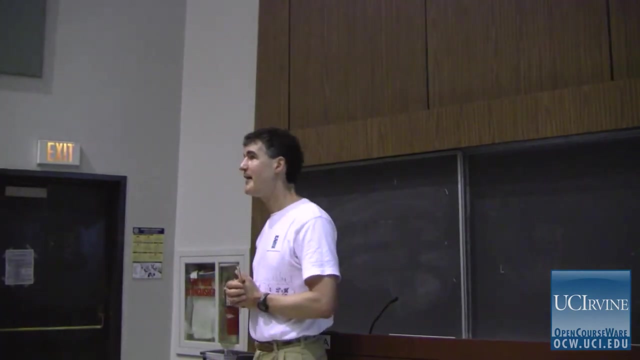 and not surprisingly, just to balance chemical equations. okay, let's talk about heat capacity. I think probably the last time I had raisin toast was in college, but I do recall that the raisins are always hotter than the toast, but everything is at the same temperature. so why is it? 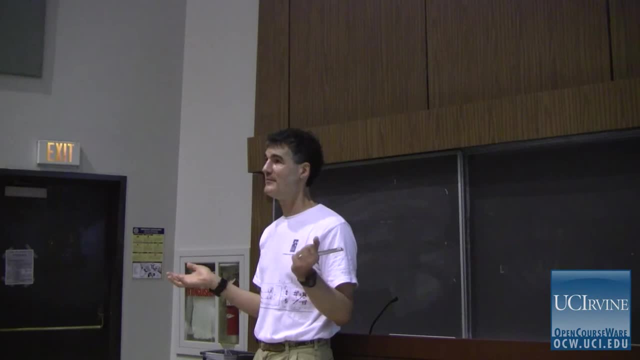 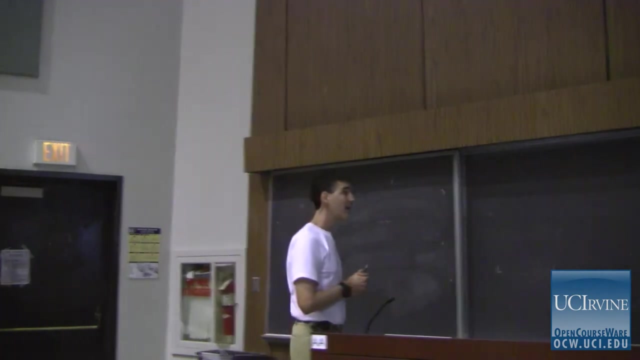 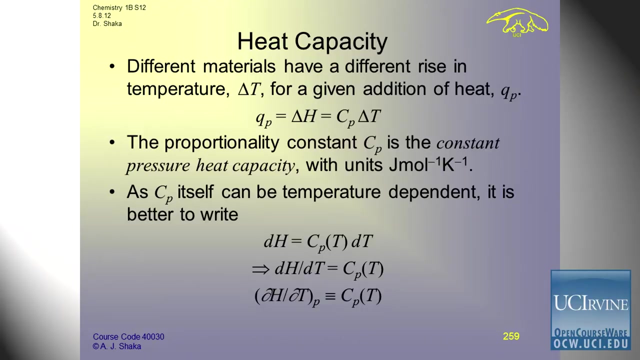 that the raisins always seem hotter, or why is it that if I get in a steam room, it's much hotter than a sauna at the same temperature? well, that has to do with the heat capacity, and the heat capacity just measures if I put in so many. 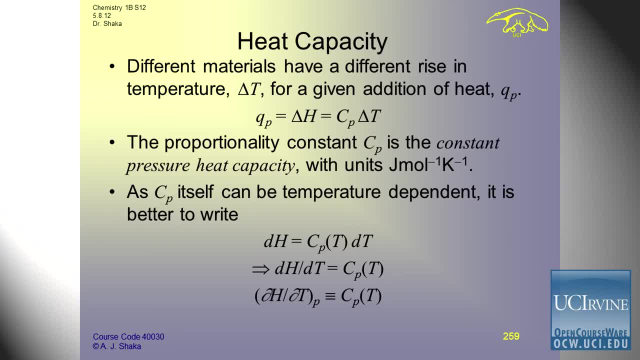 joules of heat. how much does the temperature go up? I put in the same heat. it's a different thing. the temperature goes up a different amount. some things seem to have an ability to absorb heat without actually raising temperature. all that much water, for example, is very good. 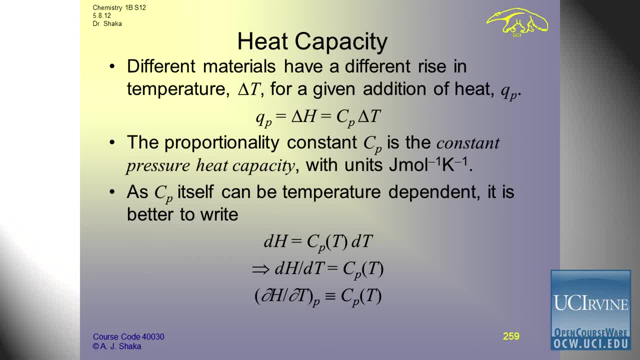 and things like that are very good to cool stuff off and absorb a ton of heat. that's why we use water to put out fire and whatever this proportionality constant is here. this C sub P is called the heat capacity and if you do it at constant pressure, 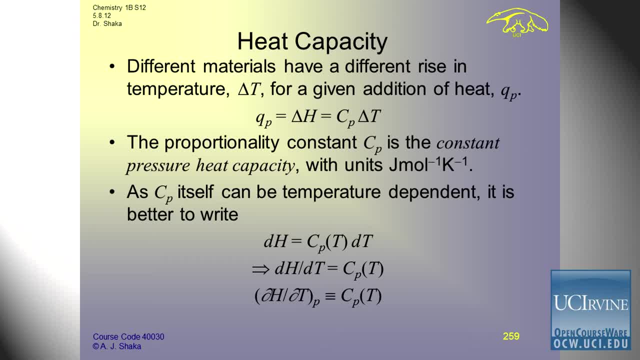 it's the constant pressure, heat capacity, and if you do it per per mole then it has units of joules per mole, per kelvin, per sideways, per degree. it turns out the CP itself can depend on temperature. it's not just a constant but it may change. 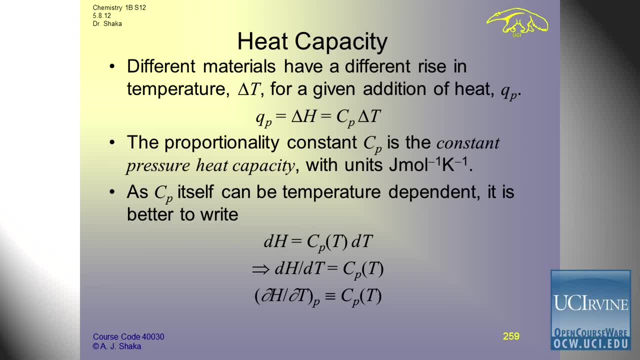 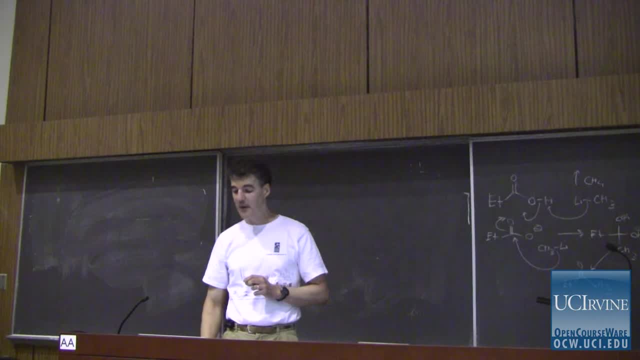 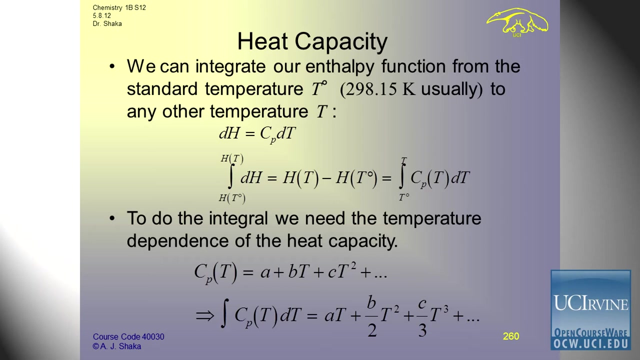 as you heat stuff up and if you want to do accurate work, take into count the temperature and the planet of C? P, and in fact you can look it up on tables things, and they just give you something like this: I start with this equation and I integrate from the standard temperature, which might be 298. I can 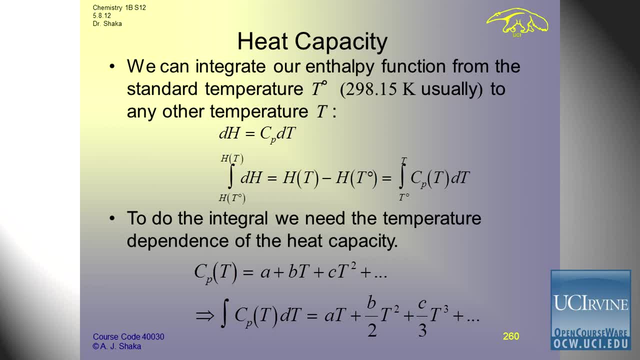 look up Delta H in the table at 298 and I can look up. I can go to some other temperature, let's say a thousand Kelvin, where I want to run my chemical process, and I can take the difference between the enthalpy state function at these two. 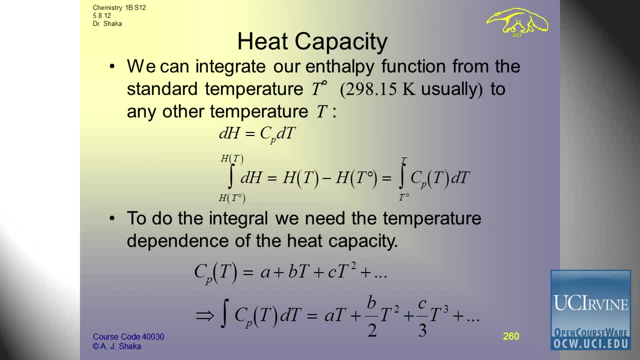 temperatures and that's just equal to the integral of CP of T, VT. so I need to know what the heat capacity is as a function of temperature, and if you look it up in books, they usually give you something like this: they say that the heat capacity of water is a plus B, T. 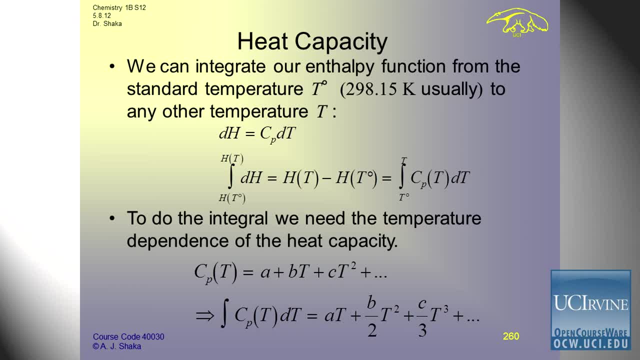 three times the temperature of water and the heat capacity of water is a plus B T. three times the temperature of water and the heat capacity of water is a plus B T plus C T squared plus, sometimes D over T, they have a 1 over T, 2 and they give you. 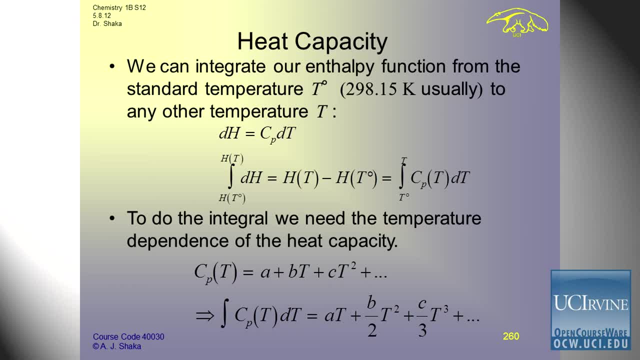 numbers here, and that means that you can shove in these numbers, you can go to integralcom and you can just do the integral and you get an expression and then, if you put in T final and T initial, you get the change, and what that lets you do is that lets you start at 298 Kelvin, where you can look up heat. 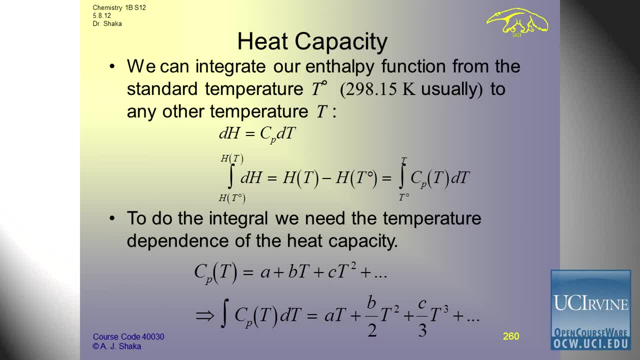 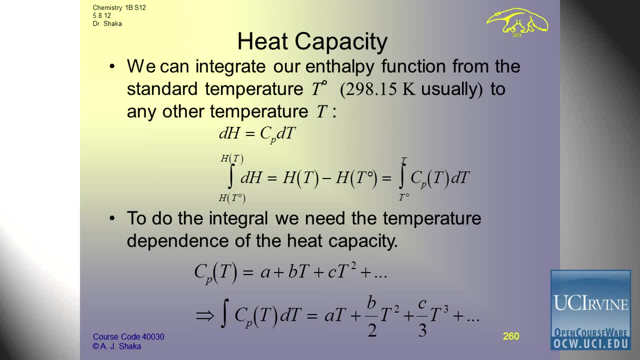 you just do it. sometimes reactions are endothermic at one temperature and then they become exothermic at another temperature. it just depends. well, we just do this trick for every reactant and every product, and I just want you to see this. I don't want you to do it. 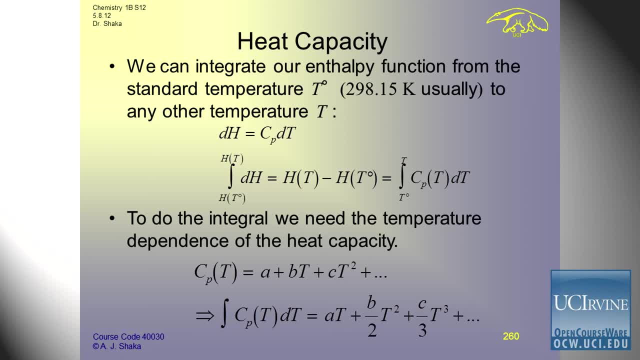 for me, but I want you to understand that you can calculate the enthalpy of any reaction at any temperature if you know the enthalpy of formation at the standard temperature and if you've measured the heat capacity of the materials over the temperature range of interest. and if you haven't, you can estimate the heat. 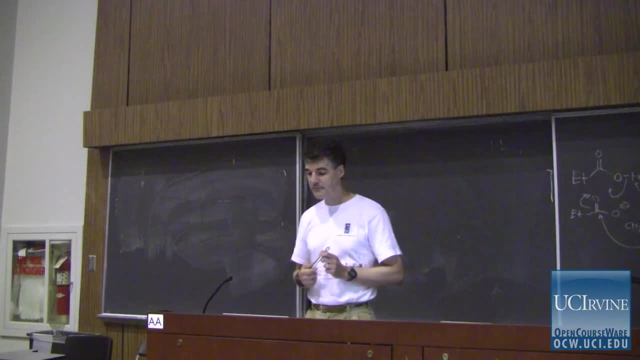 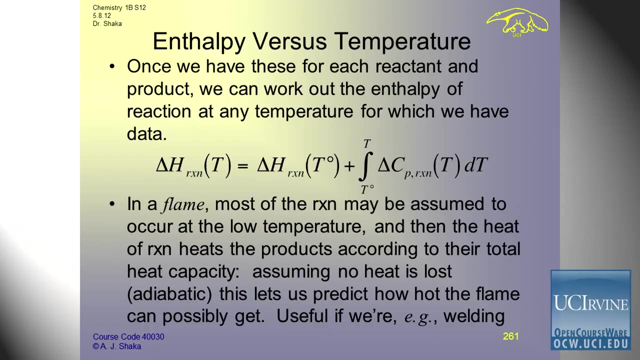 capacity. so you can still get an estimate. if we've got a flame, we've got a welding torch, we've got a flame. the usual assumption is the reactants come in at 298 Kelvin, they react and then the excess heat heats up the products. so it's the products, the CO2 and the H2O or whatever the products. 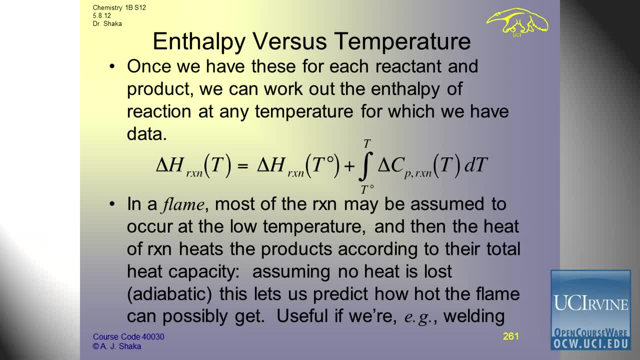 are that are coming out of the flame at the end of the flame, and then the heat capacity at the end of the flame and with that heat capacity the heat capacity extends and so, and if I know that the flame has has passed, we have the product and I assume no heat is lost when I ignite the flame. it is burning so quickly. 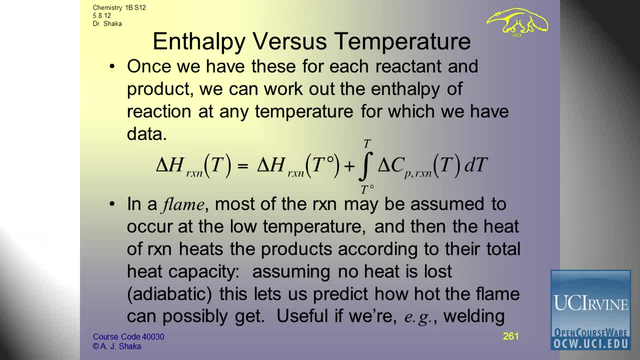 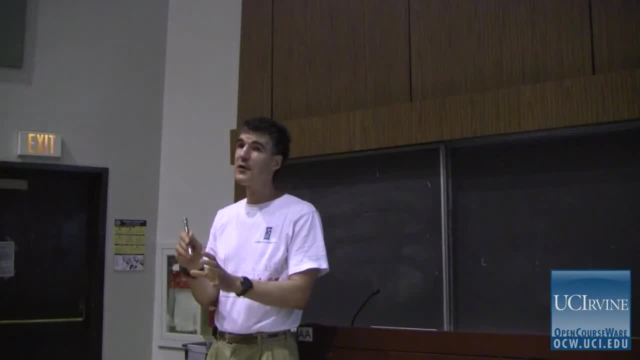 that I can figure out how hot the flame could possibly get, and that's very useful if I want to use the flame to, for example, make a welding torch. there'll be certain kind of gases that I can combine and spark it and I can get a torch and it's going to be. 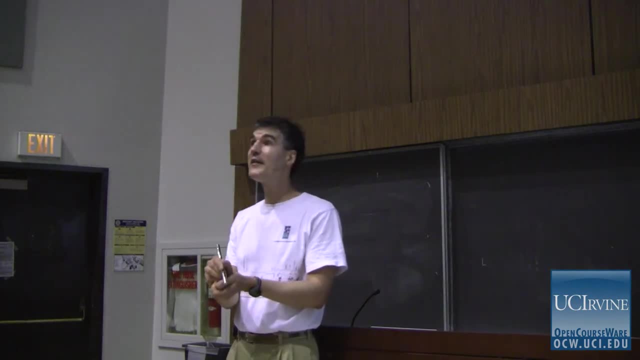 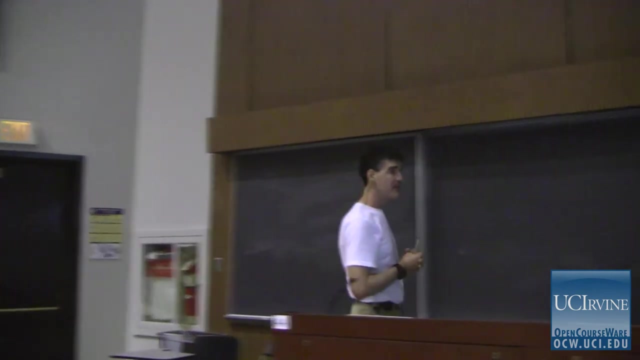 really really hot so I can weld steel with it. and there's going to be some other gas like liquid propane that if I use that in a welding torch it's not going to get hot enough to make a proper sealed, actually melt the stuff and get it to weld together. 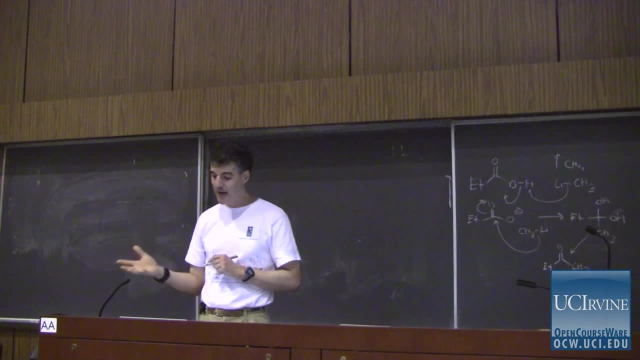 and therefore, if I know how hot I have to get it and I have a choice of buying a canister of gas, I buy the cheapest one that's going to do the job. that's the one I have on the work site, not one that goes to 3,000 kelvin. 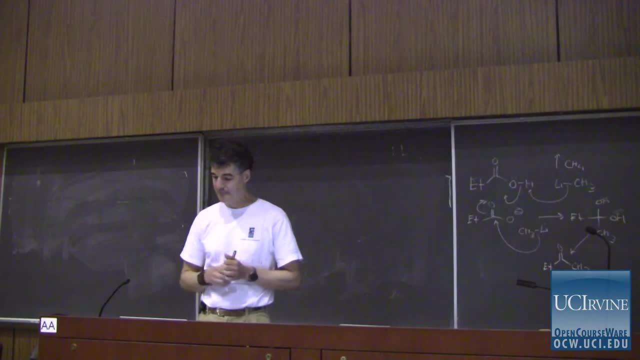 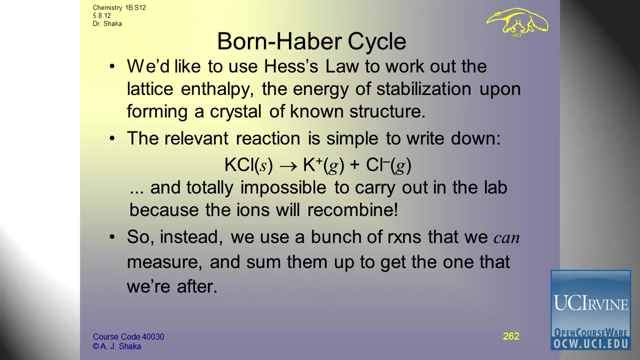 that I don't need. if I don't actually need that, okay, we won't have time to finish it, but let's just set up the, the scenario we know we can write down delta H for reactions that we can't do, and there's one special reaction that we 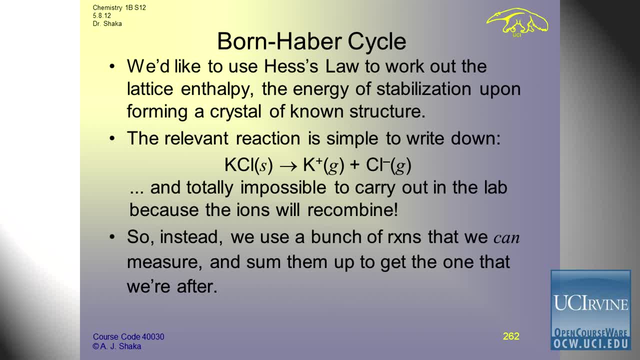 can't do, which is the lattice enthalpy of a crystal. that is of a lot of theoretical interest, and so we'd like to get a number for it, because, although we can't do the reaction it turns out, theoretical chemists and physicists can calculate what it should be. 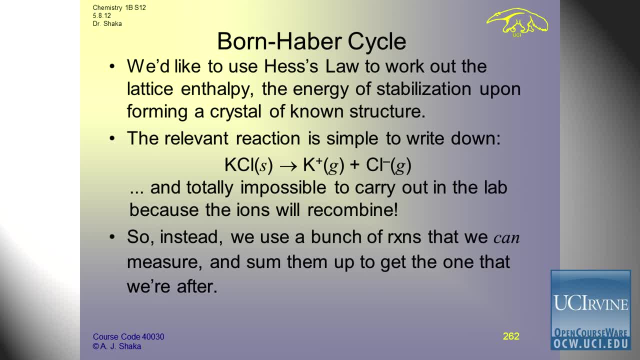 and they want to know if their calculation is right on the money agreeing with the experiment, or if their theory about how all the forces in that salt is wrong. so we want to be able to supply them with a number. and here's the lattice enthalpy. it's a very simple reaction to write down.